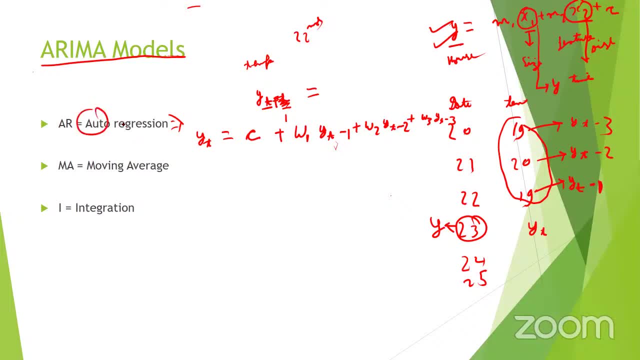 With itself, as the name is also suggesting auto plus regression, taking the regression of the term itself, right. And here now one question comes into picture that, okay, till how many previous time steps, previous data points I have to take, right? For example, here I am taking the last three data points here, right? Last three time steps data point. That's why it is Y, T minus 3, right. 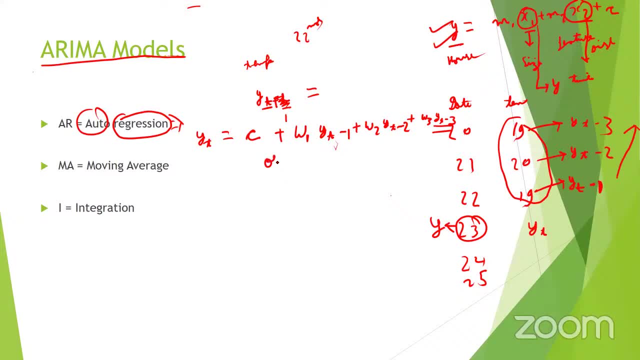 So this is my Y T minus 3.. Now, that's my Y T minus 3.. Now that's my Y T minus 3.. Now, that particular thing that will decide the order of your AR- order of AR- And that is generally represented by my P. So this P will tell me that. okay, till how many previous time steps I have to take my data points? 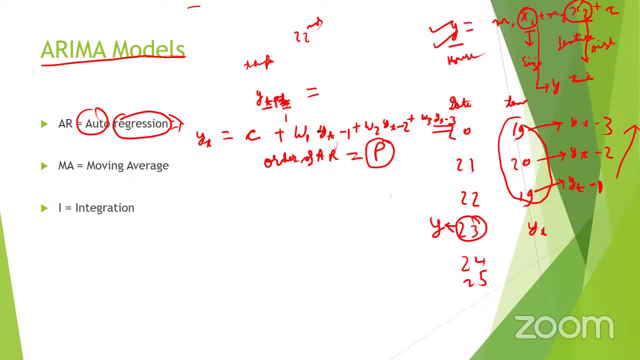 So in this particular case, my P is equal to 3 because I am taking past three data points: Y T minus 1, Y T minus 2, Y T minus 3.. So this is my Y T minus 3.. 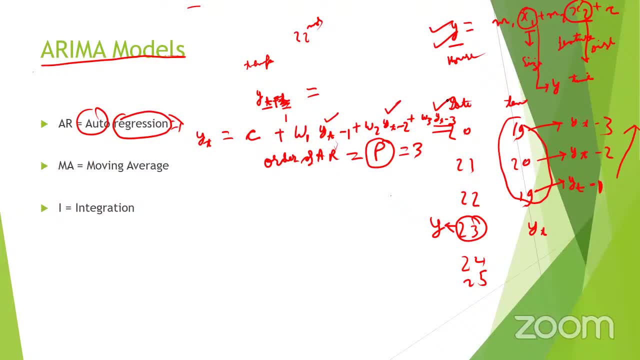 And here talking about the temperature data. but again, the same thing will be applied to your IoT sensors data also, or your stop price data also, And whatever the thing that you want to apply also will be applied on your NLP problems- natural language processing problem. 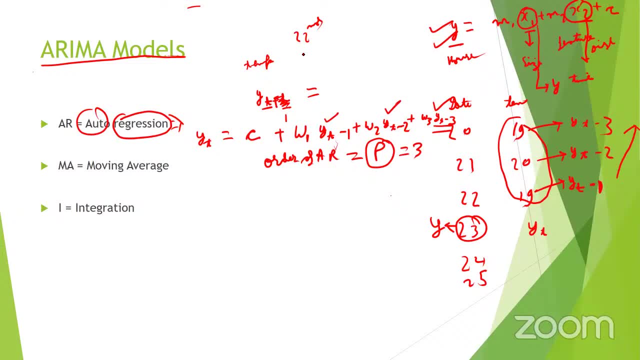 If you have one particular step, one particular sentence itself, that is again I am writing that. my sentence is: I am going to, let's say, this is my black blank space now for predicting, uh, predicting this particular thing. this will be my yt here, right? 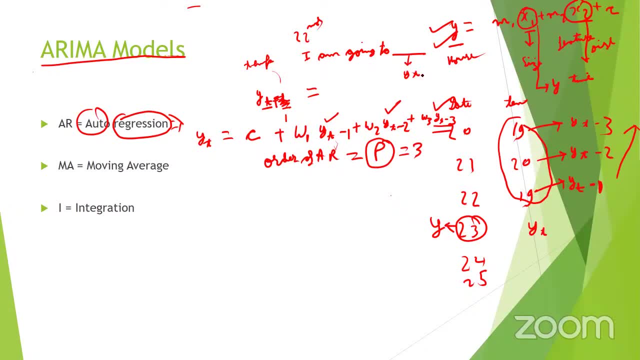 this will be my yt and my what autoregression says that this particular thing will be dependent on my last terms, right, obviously, if i have mentioned uh somewhat about that, okay, i'm 12 years old and it is the morning itself, and if i'm writing a sentence that, okay, i'm going to. 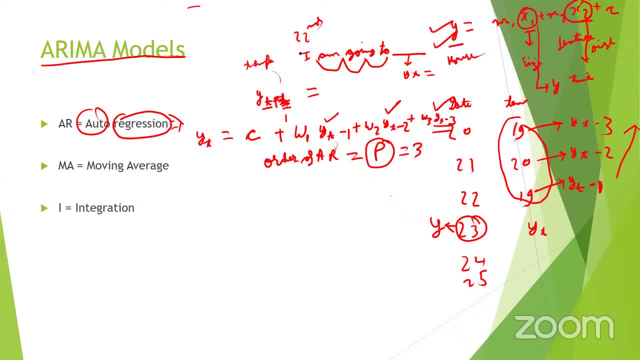 it will automatically predict that away school- maybe school will come, because 12 year old guys in the morning generally goes to school itself. so time series and nlp data are kind of related in this particular way itself. so auto regression, uh, we talked about so ar term. 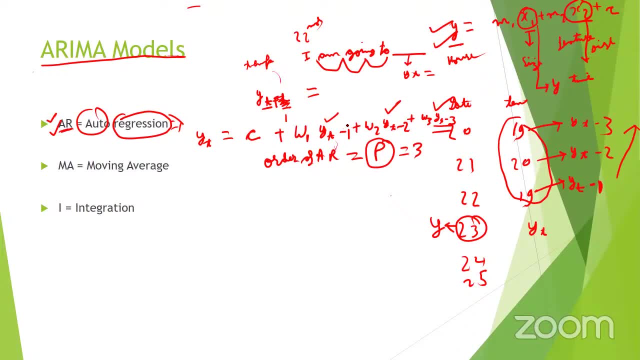 standing for auto regression, just taking the regression of term itself in my previous time steps. data next comes and make moving average. so here an average is in the picture, right? so what? my moving average says that that my value of y at a particular time, step t, will be equal to my mean of the complete data. for example- again, uh, taking this particular 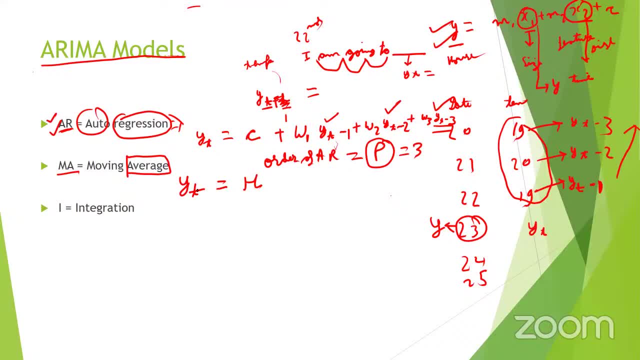 temperature data itself. so it will say that, okay, uh will be equal to mean plus c1 phi t minus 1, plus c2 phi y t minus 2, and so on. and what does exactly this particular uh terms represent that i will be telling you in a moment, and at last, one more term will be added that will: 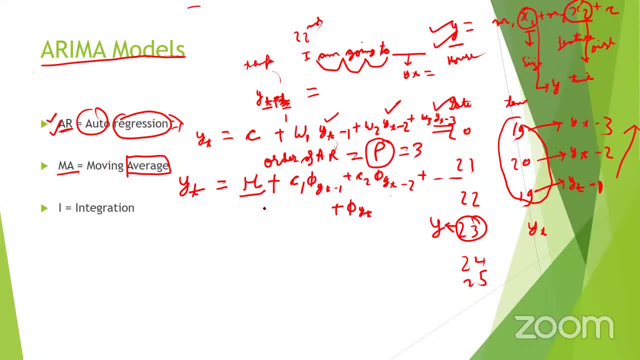 be my right point. so this mu is my mean mean of the data. so here, if you see, for this particular uh data set itself, my mean will be around 19 plus 19 plus 20 divided by 3. so it will be around, let's say, 19.4. i'm assuming that it is a 19.4 and not sure. 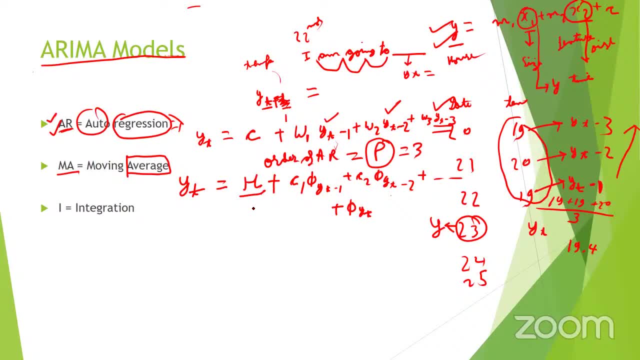 i would calculate it, but let's assume that a mean for this particular data is 19.4. so what does it say represent? how you can calculate the moving average is that your temperature for the 23rd december by 23 will be equal to this 19.4- your average from the previous days plus c1. 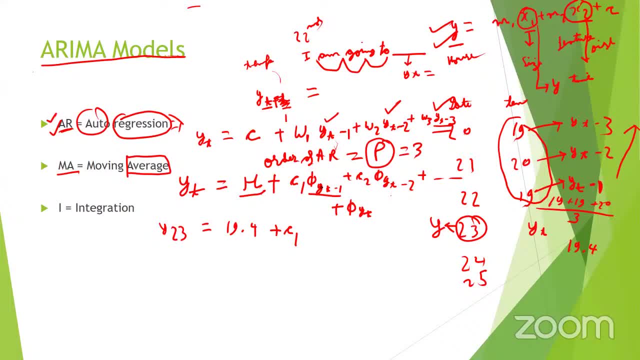 now comes this phi psi, phi t minus 1. so this psi y t minus 1 is nothing but the difference of your mean with the previous state data, right? so in this particular case, my mean is 19.4 and my y t minus 1, which is this 22nd december, is 19.. 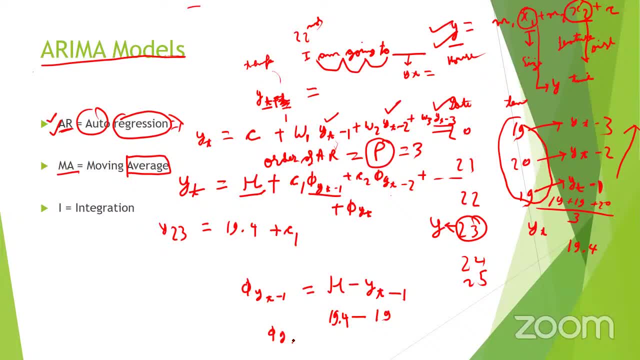 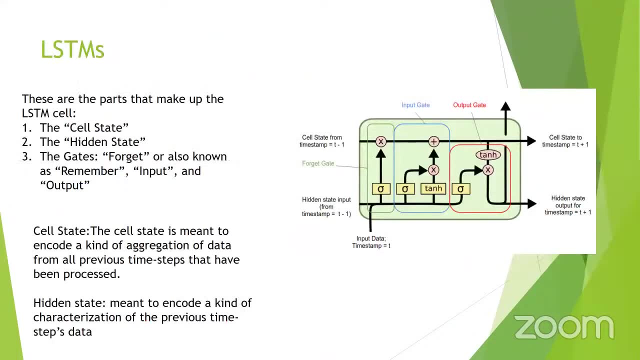 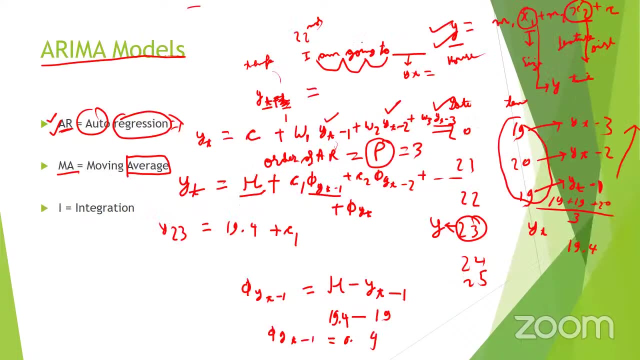 so by this, uh, psi y t minus 1 is basically equal to 0.4 itself. right? just give me a second here, just like: yeah, so this psi y t minus 1 will be 0.4 itself, right? so here 0.4 will come. now c2 and this psi y t minus 2. 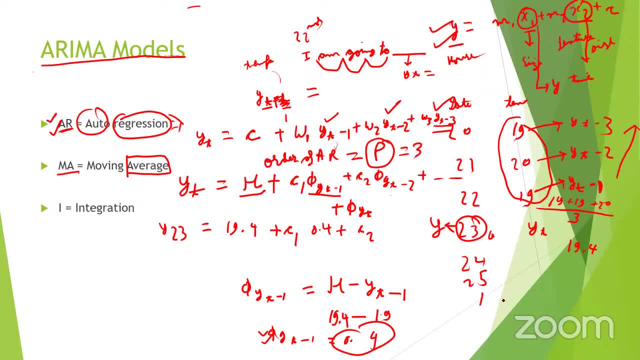 this again will be calculated in the same way: 19.4 minus y, t minus 2. in my t minus 2 it is 20, so minus 0.6 will come. in this way you will be able to calculate this: uh, psi, uh. at this moment you will have your values and you have new values now in the learning process, your. 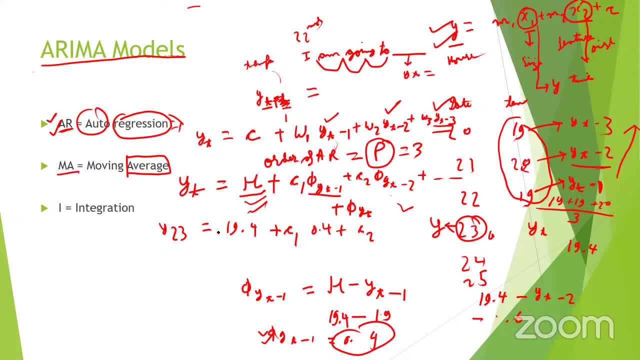 iteration process of the learning. see simply as we train the simple linear regression right by using field squared error, by using gradient descent. in a similar way, these c one, c two values will be calculated right. so this will be. this was your moving average in your. now comes integration i. what does this i stands for? 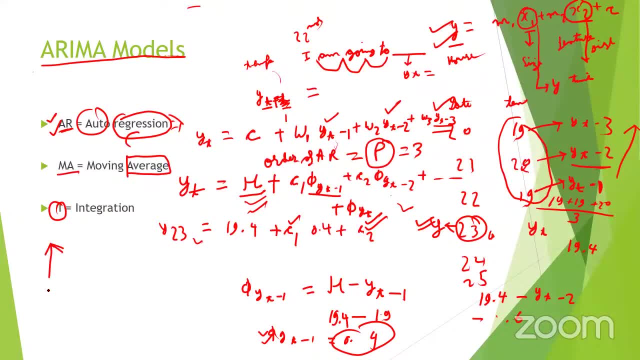 what generally happens. again, one assumption for your arima models is that your data, that data that we are talking about- need to be stationary in condition. need to be stationary in condition. so stationary basically means your mean is constant and your standard deviation is also constant at all data points. 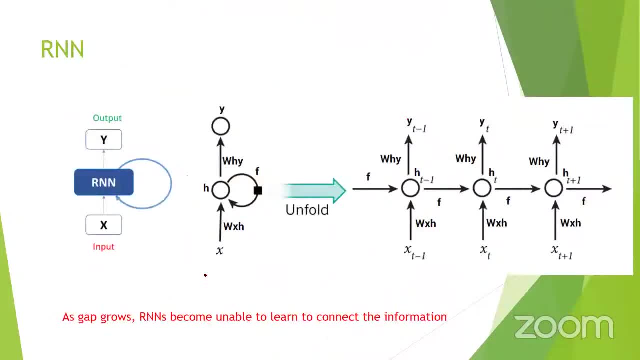 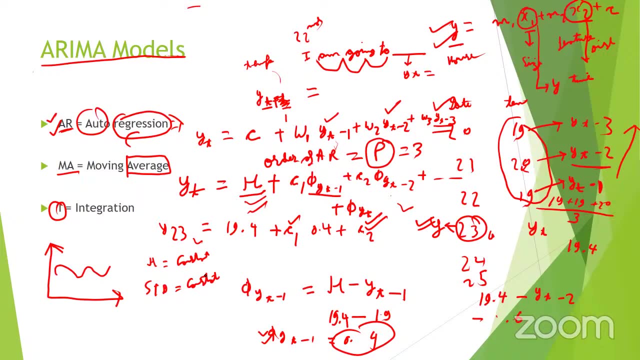 right now, if your uh, if your, if your data is not stationary in that particular scenario, your arima models cannot help you or you will not be able to use these arima models. so for making them uh, stationary, sometimes these uh, this particular thing known as differencing, comes into picture. 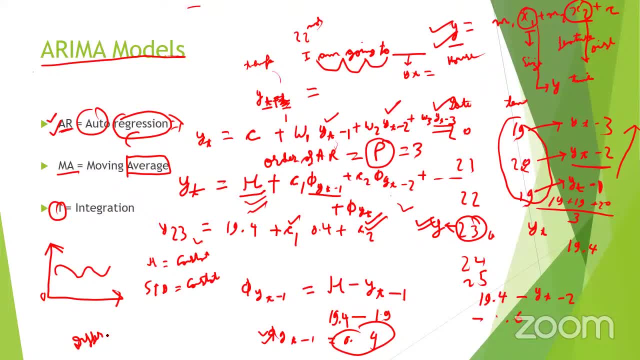 differencing comes into picture. so what exactly this differentzing is? for example, again i'm taking that i have some data, let's represent it by. while i have some data, lets again, if i take the, let's say, pressure data from a sensor, pressure data i have again for different, different types. 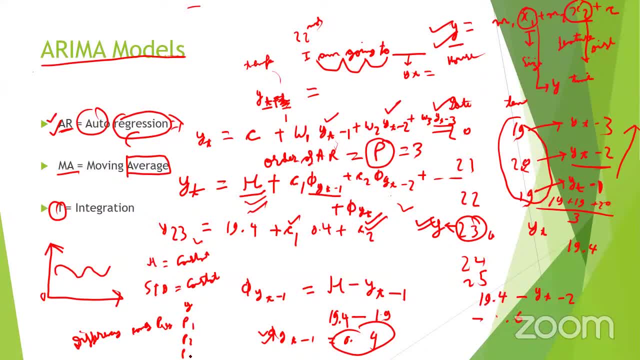 my p1, p2, p3, and i know this particular y is not stationary. after performing some of the statistical tests, i know that my y is not stationary. so what i want to do is I am going to do. I am a data scientist so I have to do some experimentation. So, first thing, what I 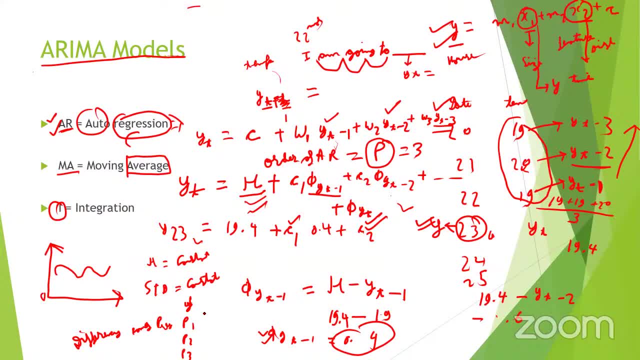 can do, I can make it stationary, I will try. I will try to see that if I take the difference of two consecutive terms, that if I take p2 minus p1 and then I take p3 minus p2, the similar way, I go on below my data points, I will take this first differentiation and again that is known as. 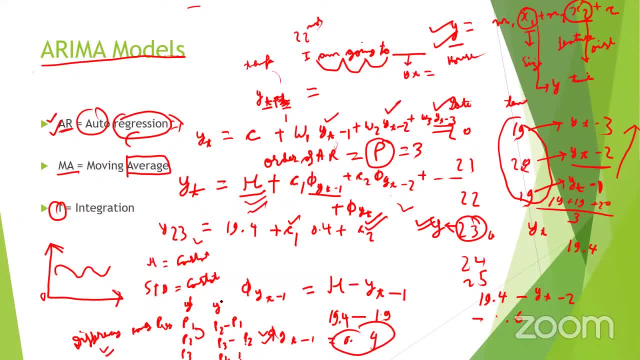 you're differencing the data and let's represent it by y dash. I have made this particular data and I will see that. okay, if this particular data, y dash, is stationary or not, and there are chances, many, there are high chances that your y dash may be sometimes from stationary. but again, 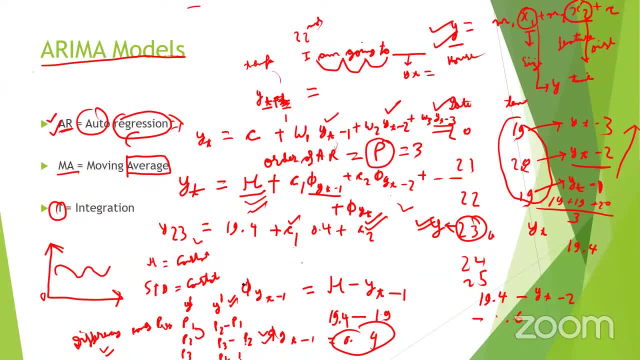 not sure, not sure is not there. there can be chances that your y dash is also not stationary. but yeah, if your y dash, y dash is stationary, then you can directly use this auto regression. and, ma on, that y dash itself, you can use directly this auto regression. 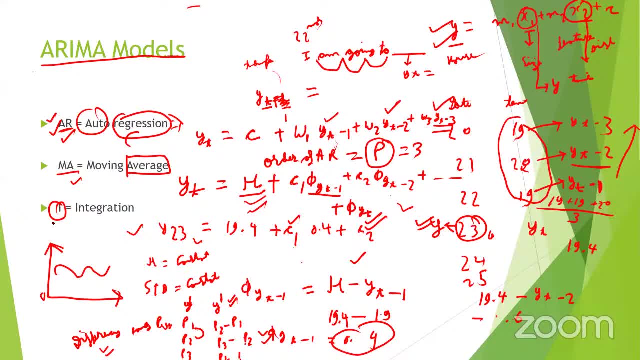 and ma on, that y dash itself. and then this i term will come into picture, because we have taken a difference of one. we have done first order differentiation, right, first order differentiation. now to get back to the original values, get back to the original scale of this y. 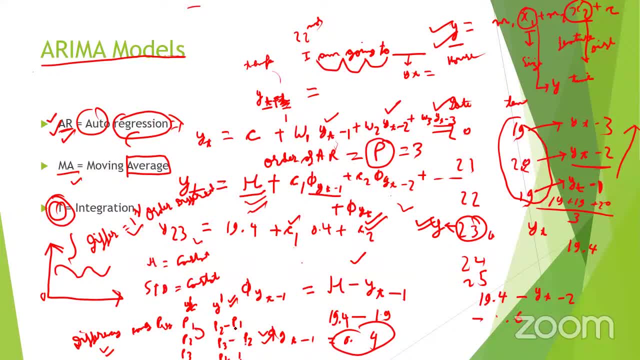 I have to integrate it again, right? so basically I have to take the previous value itself, or you can also say the integration factor. so from there, this integration, or this i terms, comes into picture. just reverse the differencing that you have done, and again this differencing will again depend on different, different orders. maybe there can. 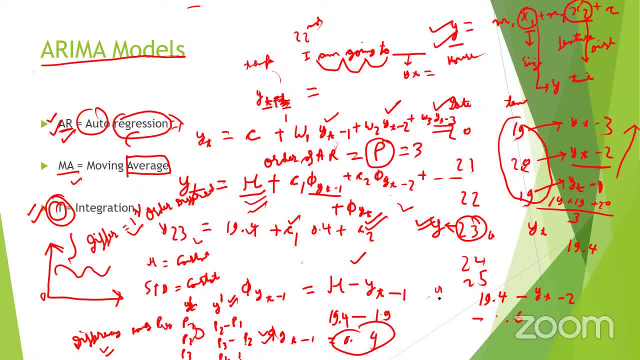 be a chance that your y dash is not stationary in that particular thing. you need to take y double dash, where what you will be doing, you will again taking the y dash, you will again taking the y dash- it means i2 dash and taking its difference with y1 dash. so these are your rima models basic. 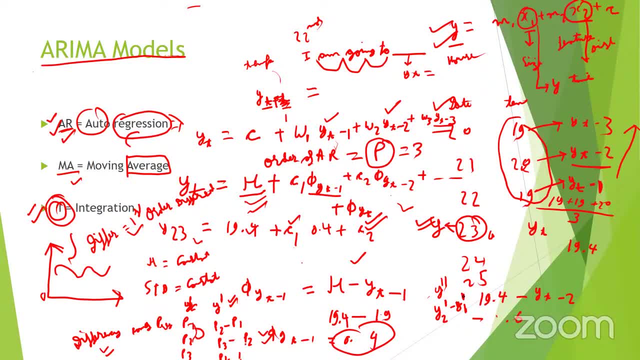 statistical models. now the problem with these models are these are: these are not able to kind of get a non-linear, complex relationship between your yt and your yt-1s right and for doing a that purpose, for solving that particular purpose. your neural network comes into picture again if we 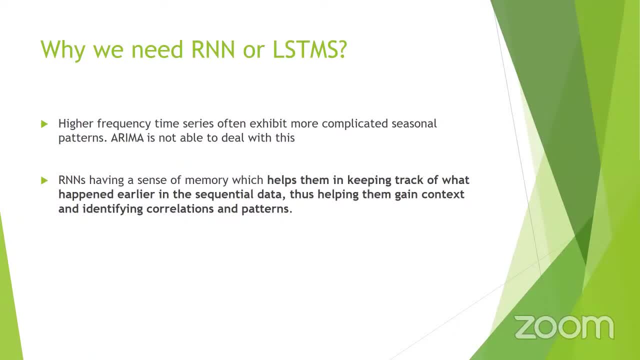 take the analogy of this time series analysis itself with the simple models, AIML models. you know that there are statistical models or shallow learning models present for simple data, random forest and all those things. But there is a scenario that if we have some complex relationship, 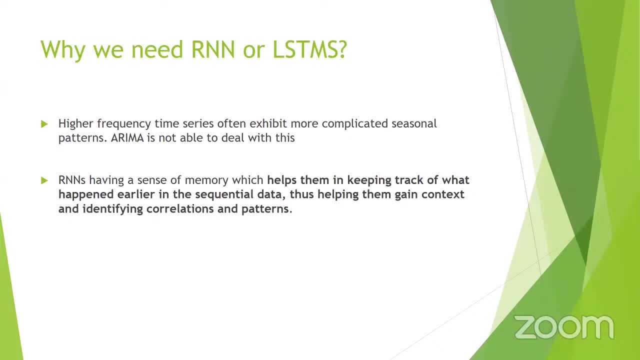 between my Y and X. we need to use neural networks because those are way better in handling the complex relationships of your feature and target variable. right Now our neural networks comes into picture. AR takes into consideration autocorrelation. Karim K is asking the. 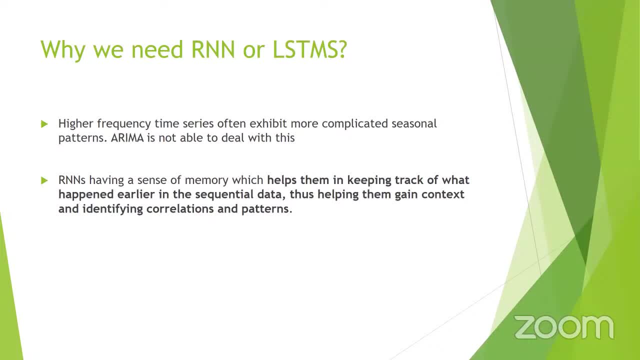 question. Yeah, AR kind of stands for autocorrelation. I think your doubt is solved Now. yeah, neural network comes into picture, but not simple neural network. The neural network that deals with the sequential data, you know, time series is a special type. 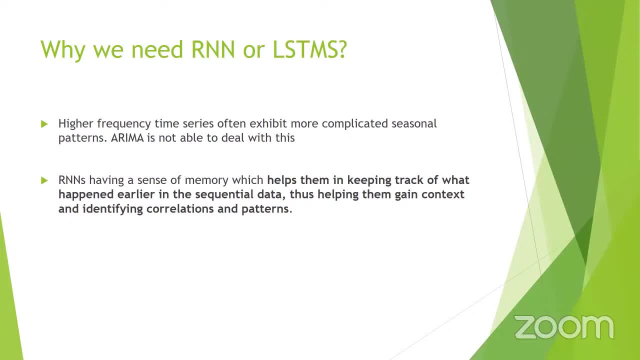 of data. right Sequence. Yeah, RNN comes into picture. RNN or LSTMs RNN. you can just say that RNN is the father of LSTM. came before LSTM, but it has some particular issues. That's why LSTM came into picture. 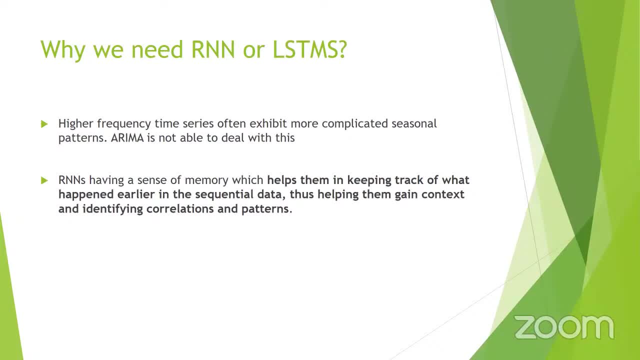 And currently, now, nowadays, we generally use transformers and all those things, But main concept behind them is sync. Now here again, as I mentioned, when we are encountering some high frequency data, you know, in our industry, production industry- 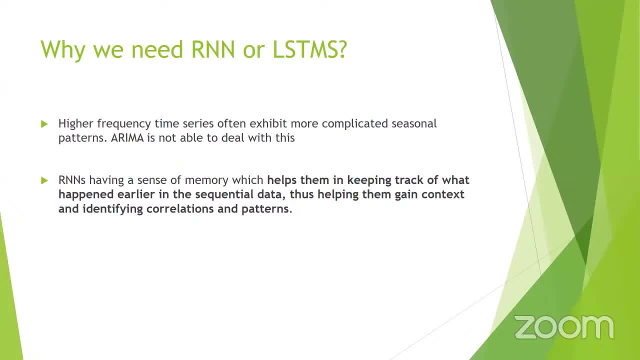 itself. if we have some sensors, data related to some equipment, there will be a higher frequency data right In those type of scenarios. your RIMA is not able to deal with that particular thing. So for solving all these problems your RNN came into picture. 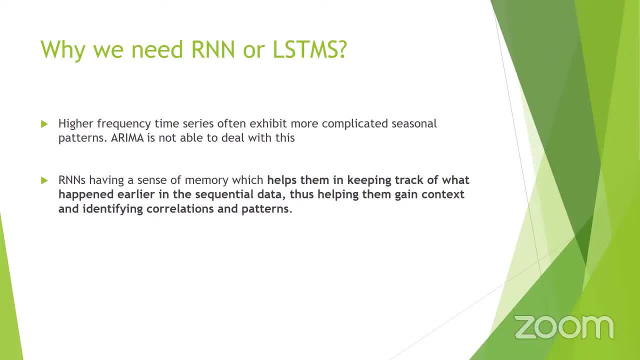 Now, first question: how RNN is different from ANN. So, as I told you as we started this session itself, that your ANN will deal with the simple data right And RNN will deal with the sequential data right. So how RNN will deal with the sequential data. 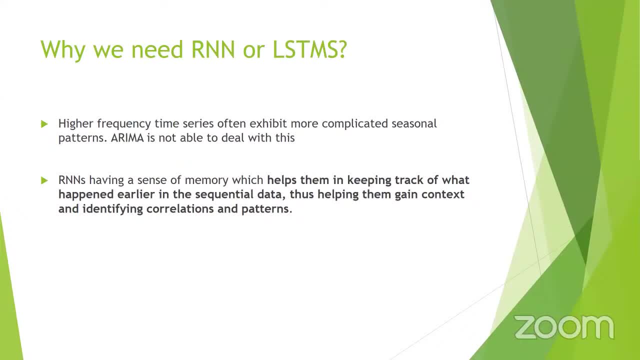 So RNN is kind of having a sense of memory. In a similar way, human beings have a sense of memory, RNN also have a sense of memory. Using that particular sense of memory, it will remember that, okay, something has happened. 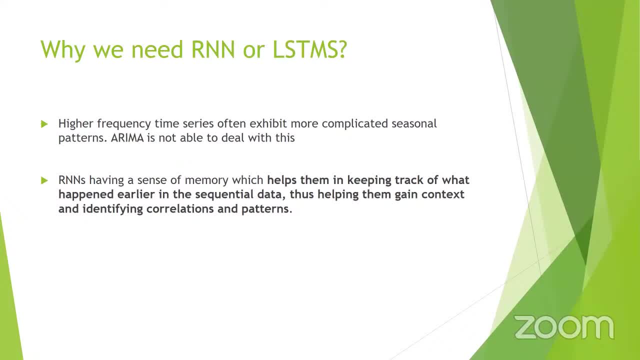 several time steps before And when we talk about the ANN. in ANN, this time dimension is not even present there. We are just talking about point-to-point- you can say point-to-point operations, So time dimension is not even present there. 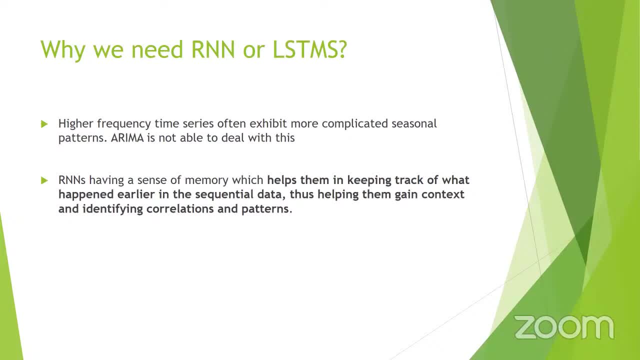 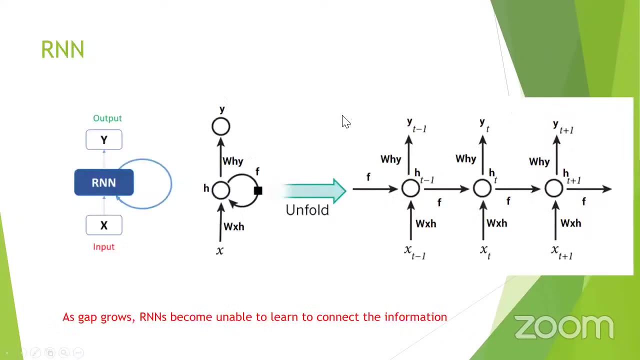 So in RNN there is this sense of memory that will help to get to previous data right And give you an output. And again we will see in mathematical terms also how RNN will deal with the sequential data And in mathematical terms also how all these particular things work. 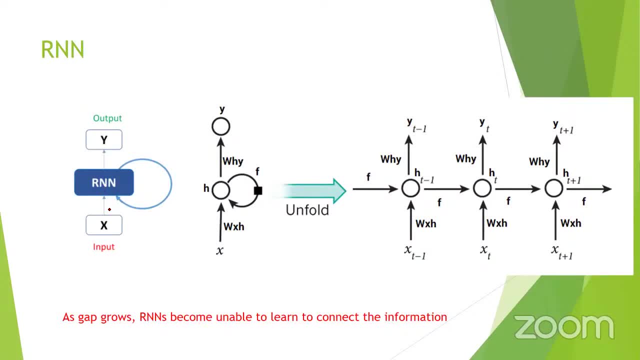 So this is your basic structure of RNN. Here, if you see, I am passing my input inside my RNN and it will perform some operations, some mathematical operations, right, I don't know what mathematical operation it is performing at the moment, but it will perform. 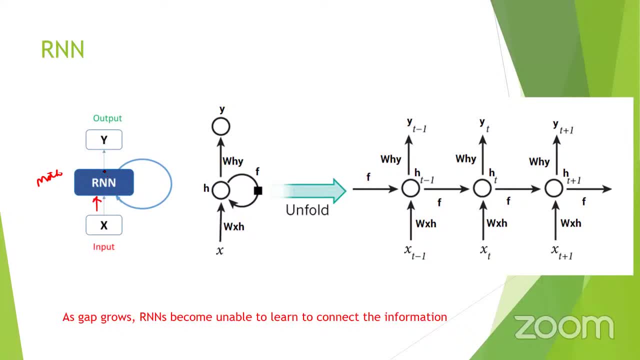 some mathematical operations on my input data, And after that it will give me an output Why And what it will do. it will also feed this particular encoded data to itself again. Now, if you unfold this particular RNN here, let's assume that I have designed a neural. 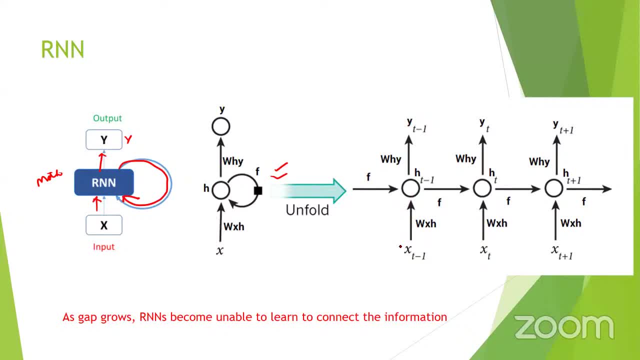 network that will take last three time steps of data: xt minus one xt and xt plus one right, And here one RNN layer is present. So what exactly is happening in RNN is first of all this xt plus one. 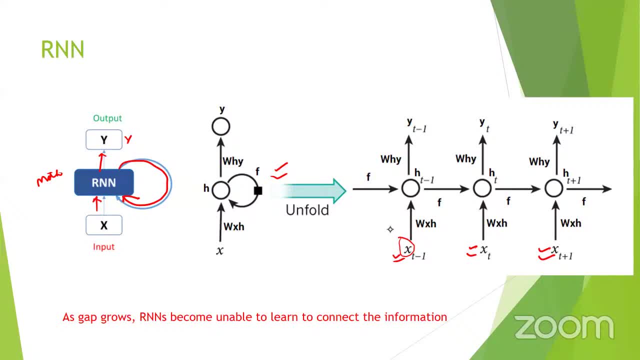 Right, Right, Right. So this xt minus one will be encoded, or your feature will be extracted from this xt minus one and it will be converted to some other state, known as hidden state, of your neural network, represented by this xt minus one right. 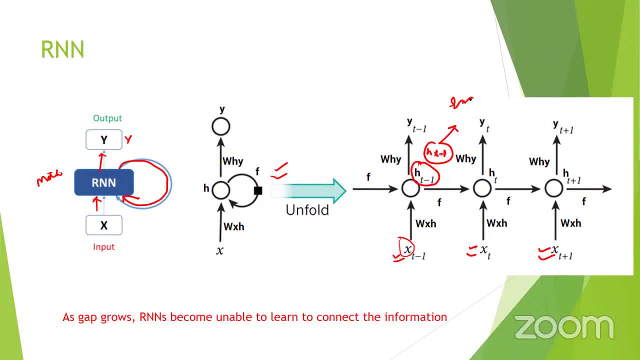 Now this is your encoded data, Encoded data that is useful for your LSTM, for learning the feature, right. And now, by using this encoded data, again mapping, because you know neural network at last will be doing the mapping between y and x, right? 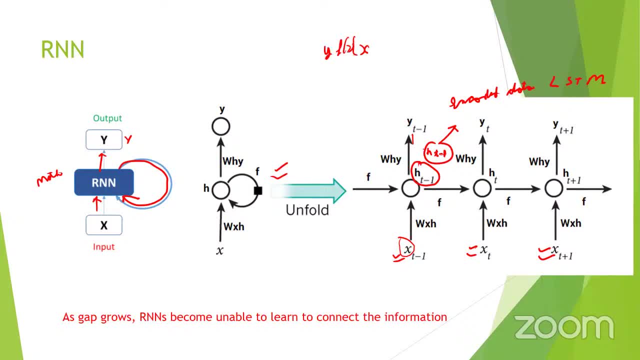 y and x. it is trying to find the function between them, right. So we will get this yt minus one from this xt minus one, But also this hidden state of my t minus one data point will be passed to next time step, also right. 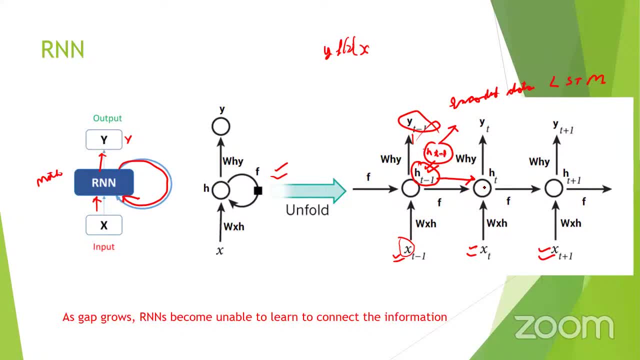 So when I am trying to, or my neuron, when this neuron is trying to get a relationship between my xt and yt, it will be passed to the next time step. also right, So it will also know this xt minus one from my previous step. 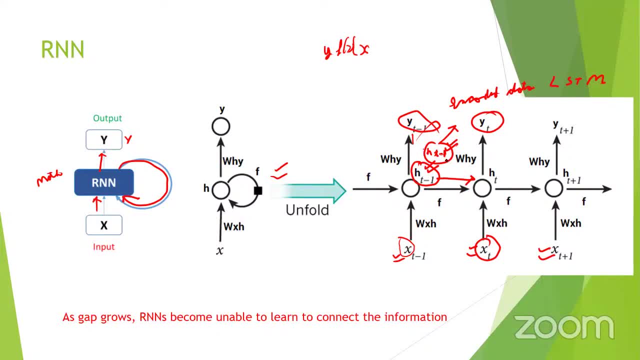 So it will also know some of the relationship that is imported inside this xt minus one that is storing the information over the previous time step itself. So it will get to know that, okay, something is happening in my past and that may be, or. 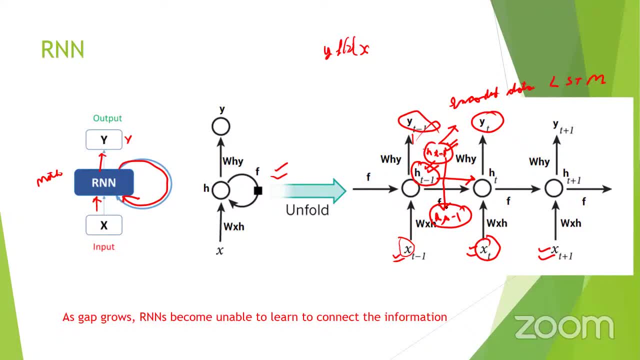 may not be useful for predicting my future. So in this way, your simple, basic RNN models will perform right now. but the main problem with this rnn- simple rnn model was it that there was some loss of information there. if we go uh deep or if we go back a lot in the past, it was not able to remember. 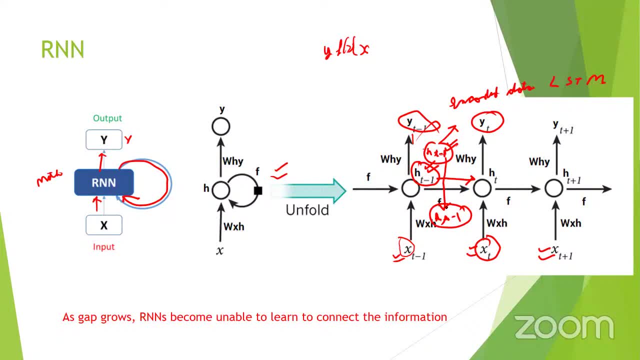 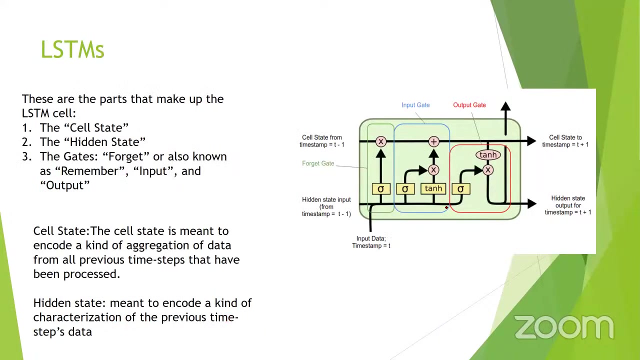 the stuffs it have. you can say it is having short memory issues. it doesn't have long memories, right. so for solving that particular scenario, my lstm came into picture, right, and how lstm works, or what is the, yeah, what is the uh inner structure of lsdm? let's say so for solving that particular. 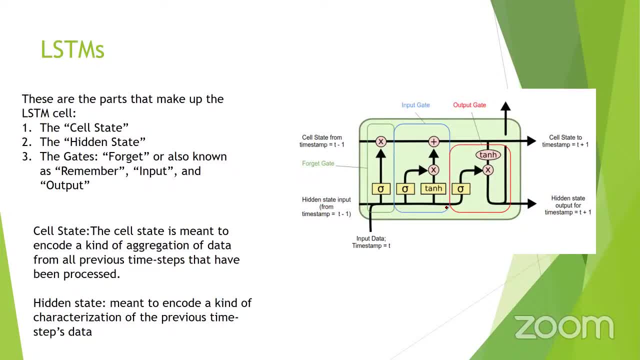 long-term dependencies of rnn. lstm came into picture and here, if you see, in lstm there was this hidden state, right? so, apart from this hidden state, one more thing was: uh, and it inside my lstm, that was this cell state. so this is a basic order. you can say, this is a basic. 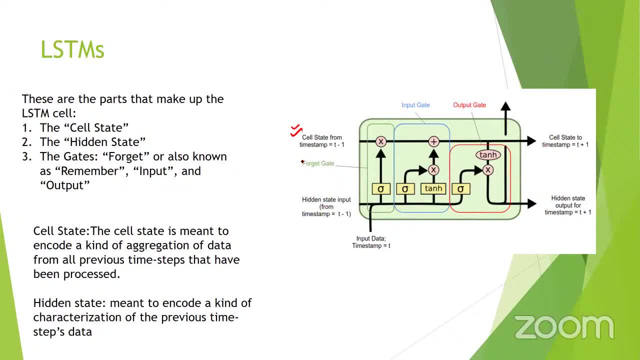 structure of one of your lstms and how it looks like, right? so i will be explaining one of uh, all of these units itself that constitutes your complete uh lstm itself, right? so there are three different things. three different parts make up your lstm cell. one is your cell state. one: 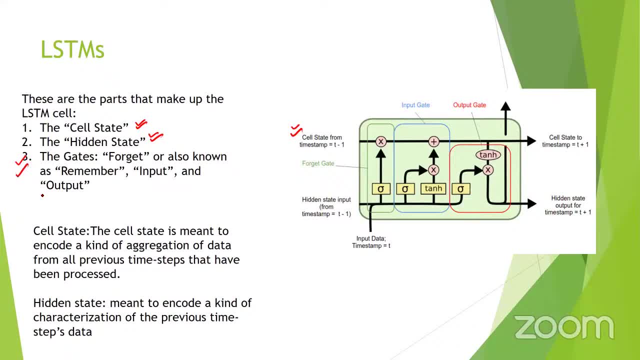 is your hidden state. and the third one are your different, different gates, right so, cell state. you can say that cell state is nothing but the complete memory of your lsdm cell or your computer lstm network. you can say that it is the memory of your lsdm network. 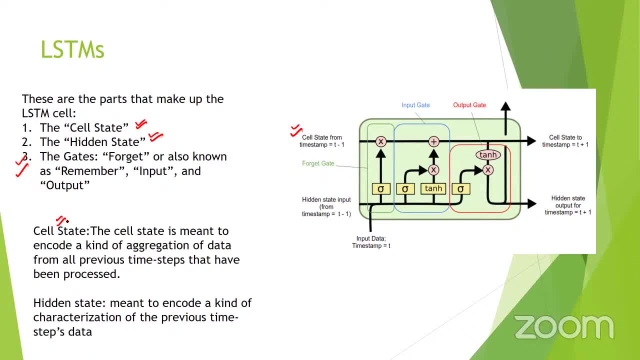 it is the thing that is storing the information of the complete data, right? or it is in an encoded way, not exactly right? so, cell state, you can say it is concerned with my complete data. so all information, all information will be stored inside this cell state, again in an encoded way. and body data, right, not exactly. and how this cell state will be calculated. that 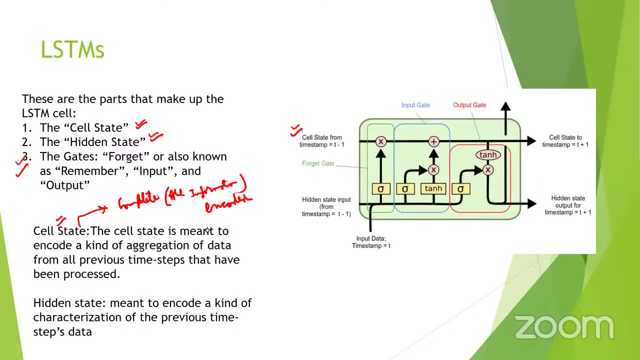 again will be uh, saying, and this particular cell state is affected by your different, different gates, your input gates, and forget gates. because, as we go on adding more and more data, we need to decide what data we need to remember from my past and what data we need to forget that particular 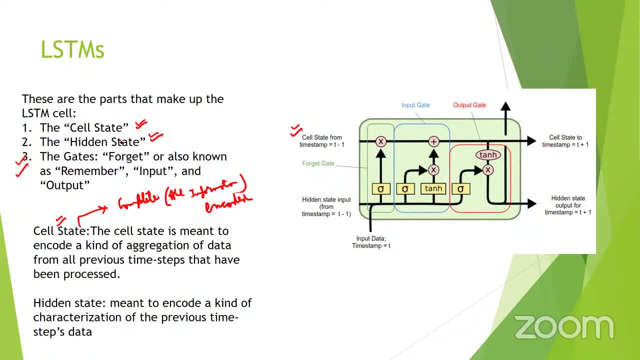 thing is your forget gate, and if we add new data for the next time steps again. we need to, again, we need to take a decision how much of that particular data i need to remember and how much to forget. so for now, just remember that your cell state is: 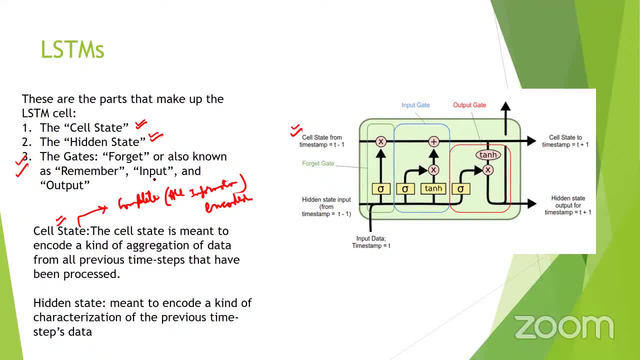 kind of associated with your complete data itself. it is storing the complete data in form of your uh encoding structure. right, complete data is stored in encoded structure and the other one is your hidden state. your hidden state is kind of: your hidden state is kind of more concerned with the previous time step only, right? so if i'm talking, 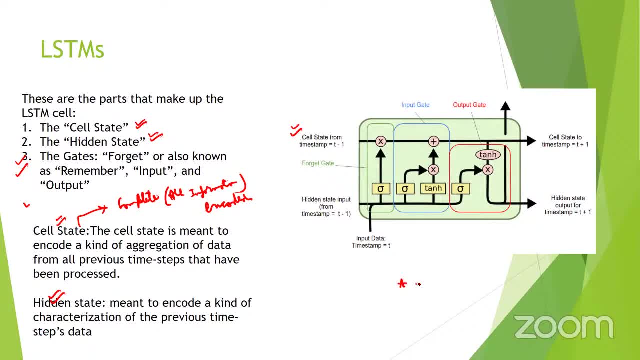 about uh. let's say t, let's say i'm talking about t. right, so this hidden state will be storing the information from my previous uh, previous cell itself or previous time state itself, so it will be having the information of complete t minus one. in one way, this cell state and hidden state are: 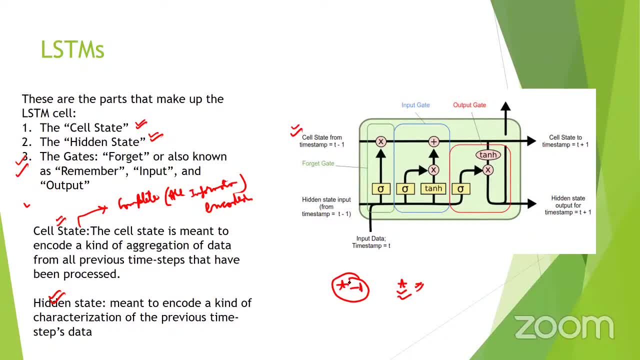 kind of interrelated with each other. again, we, when we will be seeing the mathematical things going on behind you, will be able to get an intuition of how these are, how these are interconnected with each other. but for now, just remember, hidden state is for your previous time. 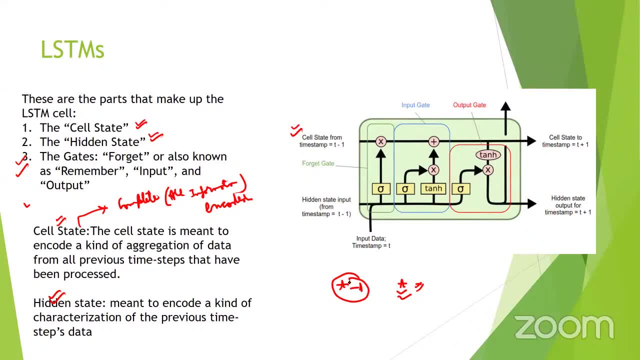 step only. so you are concerned with the recent time step right, the just the time step that has happened recently. and again, this hidden state is not equal to the output of one particular cell. again, it is the encodation of your recent type step data right. so hidden state i'm. 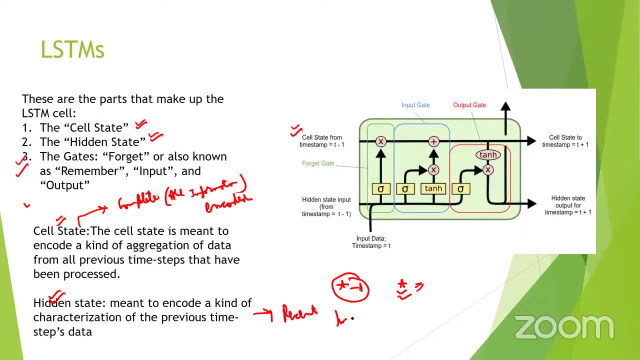 writing here recent time step and cell state from all previous time steps, all previous time steps. so what exactly happens? here again, let me make it my white team, uh, let's say white t only. well, i'm giving my y t minus one. i'm giving it y t minus two, i'm giving y t minus one and i'm giving my y t and i'm trying to map. 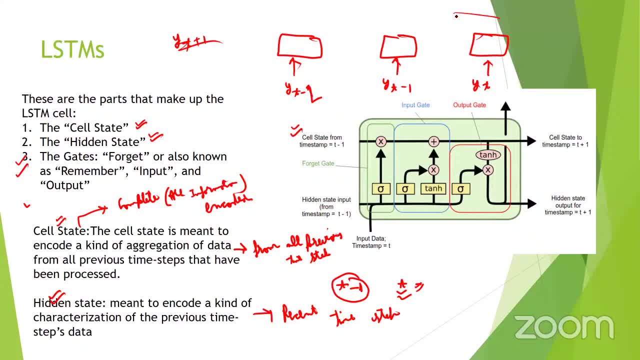 there is a complete, let's say, architecture of my neural network, having lstm cells between it. that is trying to get the function. what function? my y t plus one is equal to function of my y t, y t minus one and y t minus two. and let's say this: y t minus two. 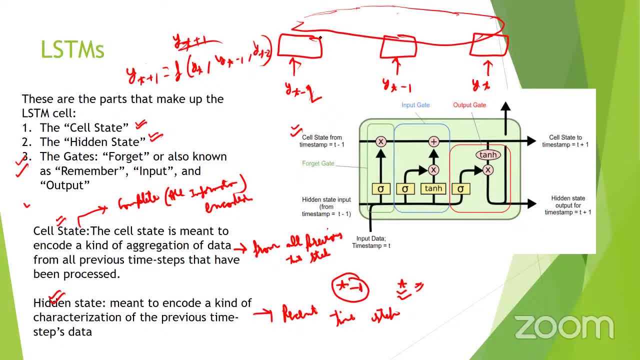 minus one and y t. these are combined, are directly connected to your lstm cell. so these are my lstm cells, so these will be interconnected with each other. also that your previous time step data will be passed on to next time step data. now, when we kind of remove this cover of your lstm cell inside your lstm cell, look like this: so there here, this is. 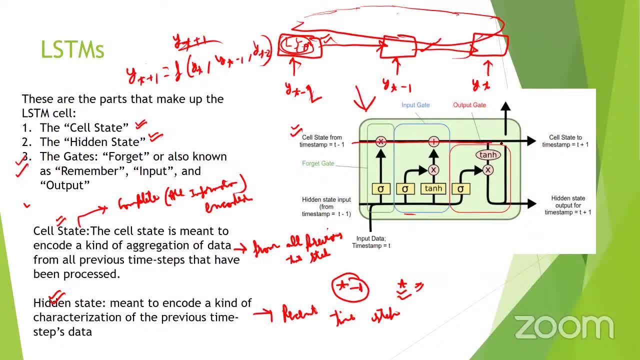 there is this horizontal straight line running out of your lstm cell. just assume it is a conveyor belt- some of the conveyor belt going through your complete lstm cells that are connected together. this is for my y t one, because it is getting the input data at time. step t itself, right? 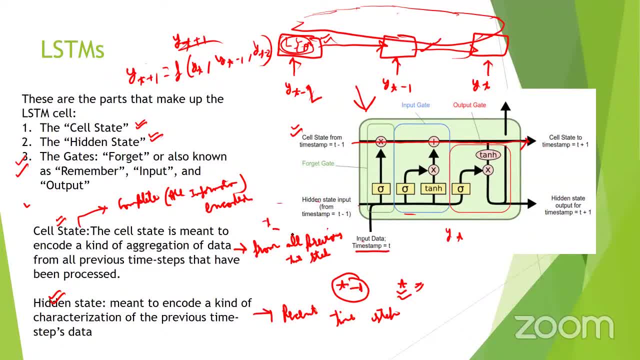 previous one. the cell before it was for t minus two, so this conveyor belt or your cell state is coming from that t t minus one itself. so t minus two is t minus one, and before t minus one was t minus two, right? so this cell state will have information of your data from previous uh. 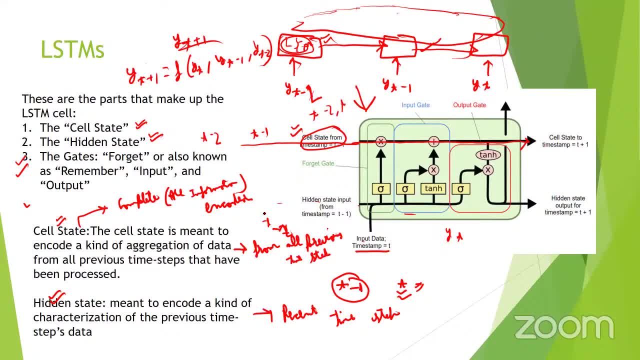 both the data points t minus two and t minus one, and the hidden state that is coming below will have your data from t minus one itself. now this horizontal line is your cell state, again a conveyor belt type of structure, having complete information. this particular green box is your forget gate. it will decide that what. 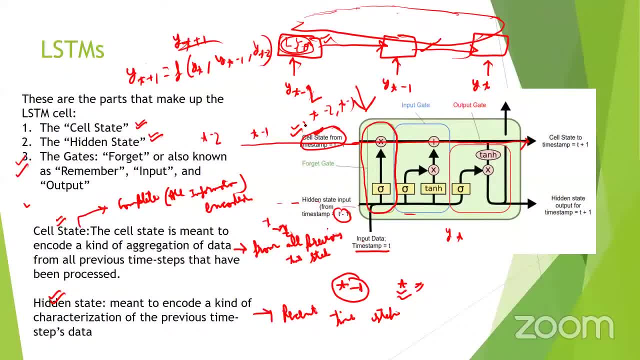 information that i am getting from my cell state for my previous cells i need to remember and what information i need to forget. how it will do, we will see. so this is your forget gate dealing with historical data for previous timestamp data, previous time step data- what to remember and what to forget- that 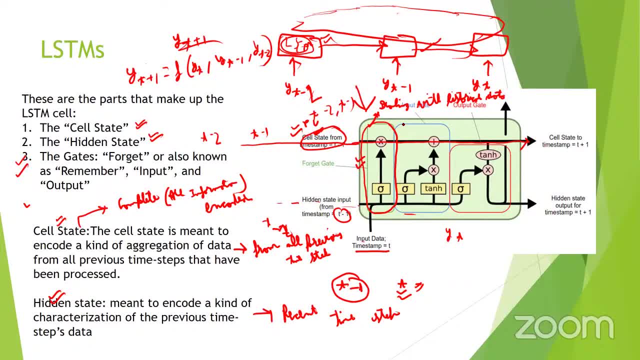 will be handled by your forget gate. next, this blue box is your input gate. now, this input gate will decide that from the current input, the input that i'm getting for my time, step t, how much i need to remember and how much i need to forget. and again, all this remembrance and forgetness, all this particular data, will be stored inside. 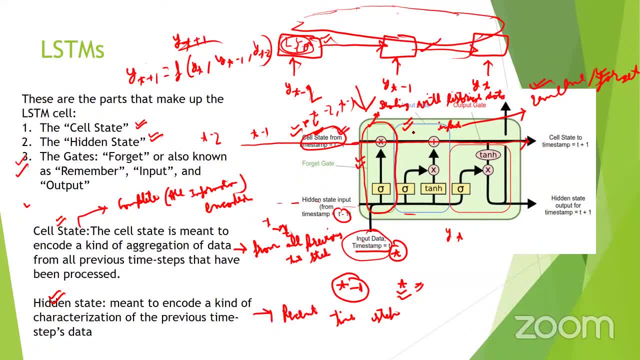 your cell state itself after some of your mathematical operation. so this is your input gate, deciding on your input gate. input last is your output gate. so output gate is responsible for giving the hidden state to the next time step. so here, my next time step, it is straight yt plus one. so giving that hidden state. 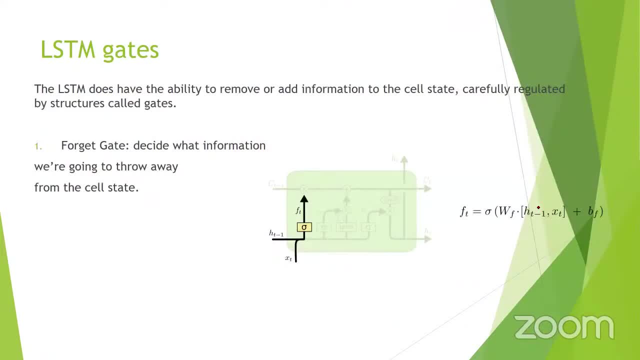 to next time, step right. so now let's get into the gates itself. so first one is my lstm gates, first one is my forget gate. right as i said, it will decide that total. what amount of data, what amount of data? instead of data, let's say encoded data. encoded data that i'm getting in form of my ct minus one. 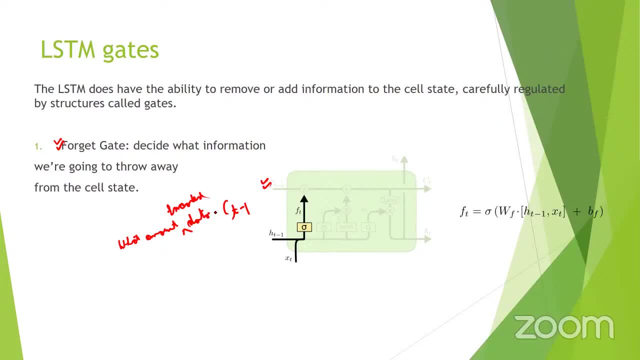 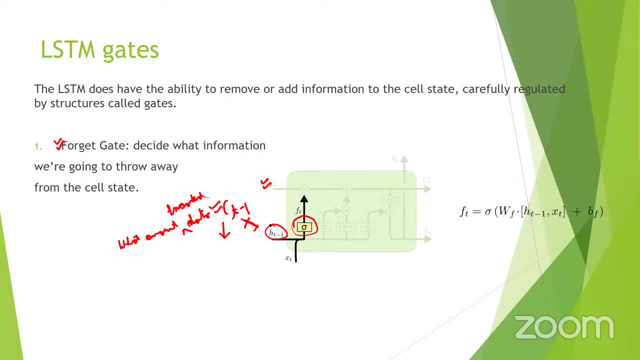 decide here. you see that this hidden state from my previous cell is coming and my this uh, current features for current time. step t is coming and now this particular operation is concatenation. so i'm concatenating this hd minus one and xd together, and here a matrix will be formed, here and that. 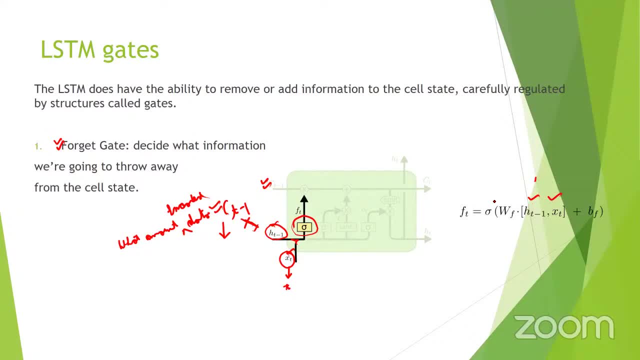 particular thing. simple, your simple neural network operations. multiplying that particular thing with your weights, this is your weight wf. wait for forget layer. right then add the bias in that particular term, again bias for your forget layer, right now. this complete operation, this complete operation will be passed through a sigmoid activation function. why sigmoid activation function? because 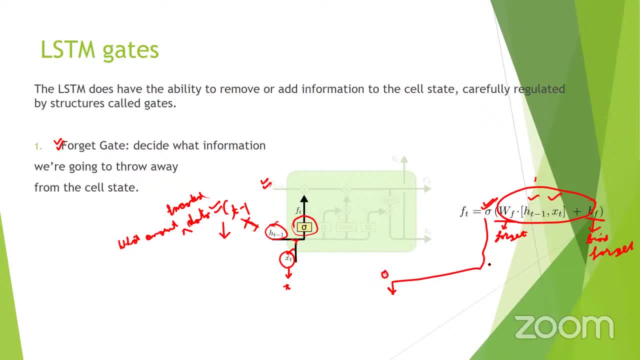 it will give me output, output in term of my zero and one right. so if my output of this particular forget gate that is represented by ft is zero for that certain given data point inside my ct, minus one, so it will directly say that, okay, that particular data inside my cell state is not not important to remember. 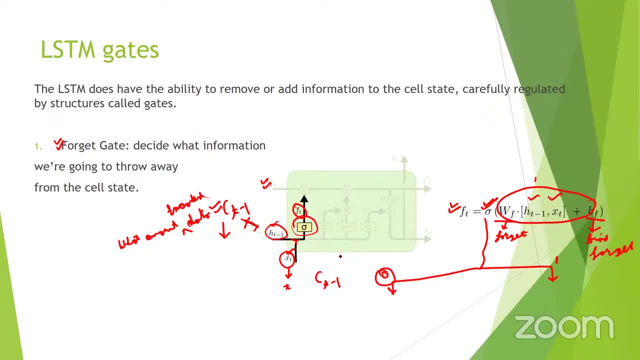 that is not uh performing, uh any, or you can say good thing, uh in my learning rate of my neural network, so that is not important for me to remember, so i just need to drop that particular thing. so it basically means that that, depending on my current state inputs, 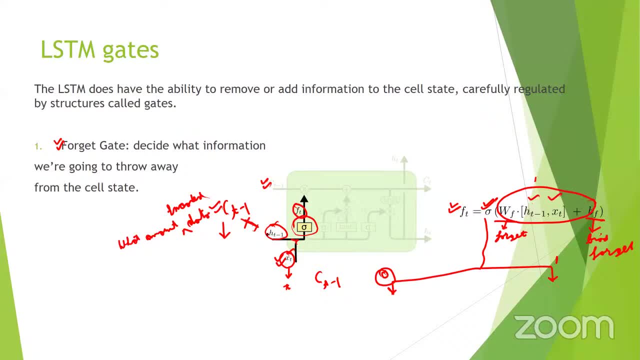 xt, depending on my current state, input xt and hd minus one. obviously i am deciding that which of my previous data, which of my previous data is important to remember, or we can just forget that particular thing. and, depending on the output of this particular thing, zero and one. i will be remembering that. 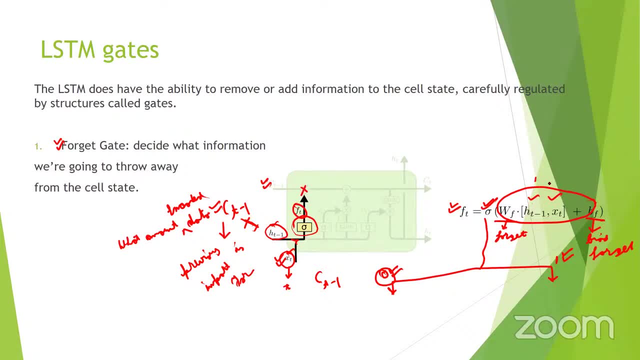 particular date on. and here, if you see, is multiplication. so once i get this ft from here, from my input gate, it will be multiplied with my ct minus one. previous cell states, whatever, whatever, either was my cell state and here it will be my ft multiplied by ct minus one. now this particular fda. 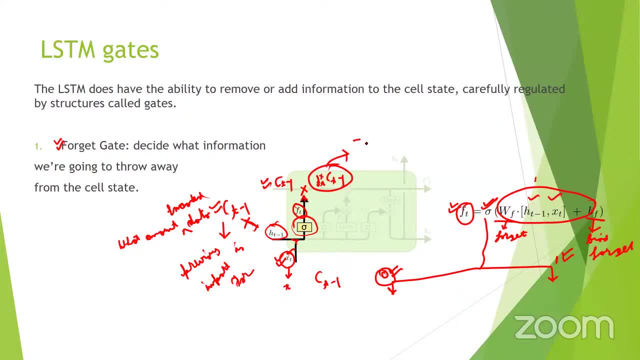 into cd minus one, only having the information that is relevant to the member. depending on my current input, current timestamp right. Ashwin is asking: go to implement the same LSTM, but the operation I want is using fuzzy. ok, now this is your forget gate, basically deciding what information from the previous cell I need to remember. 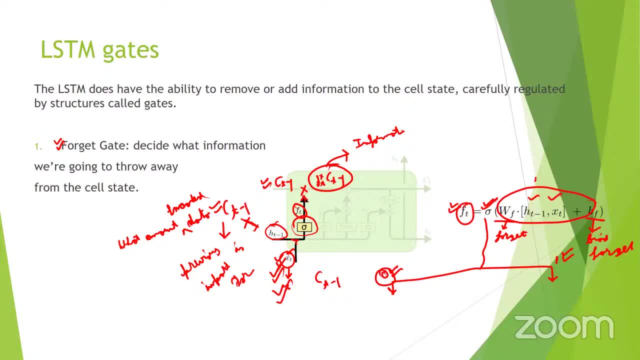 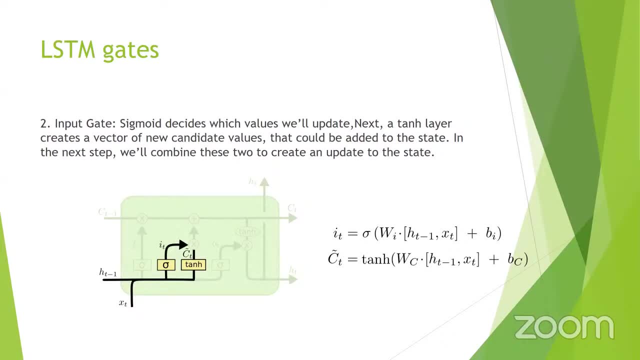 previous timestamp I need to remember and what to forget. now, coming to my next gate, that is, input gate. so my history, or past, I have handled. now come to the present. right now, this will decide here in the input gate. if you see, there are two things. one is. 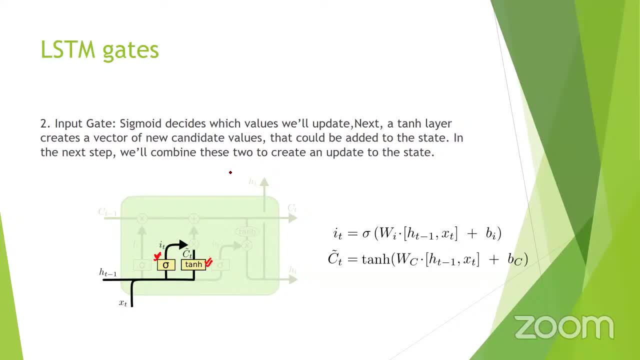 your sigmoid function and other is your tanh function. by default this complete thing is known as input gate. but there are different, different notation also where this particular sigmoid function, this particular thing, is only known as your input gate and this tanh thing is known as your. 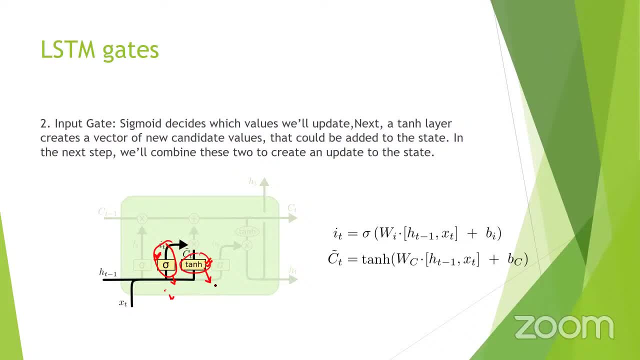 candidate. this tanh is known as your candidate gate, but again, depending on whatever nomenclature you want to go. but for now let's assume that this complete thing, this complete thing, is my input gate. now here. what will happen here if you see same type of? 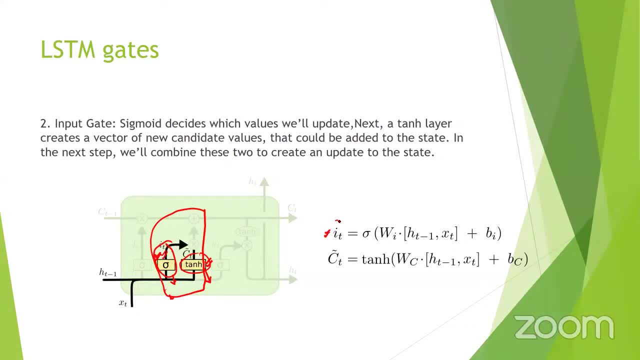 sigmoid thing is happening here, it. that is my output from here. sigmoid again. my previous, previous hidden state will be taken and my xt current time step input will be taken again, simple neural network operation I will perform. then I will pass it from a sigmoid layer. now again, this sigmoid layer will tell: 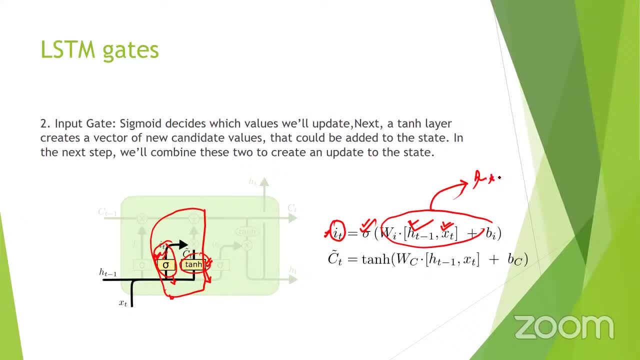 me that, depending on my previous hidden state and my current input of xt, whatever the things I want to remember from the current state, it will be taken from the current state itself and whatever the things I want to note to take in an account. so it is hidden, it is. 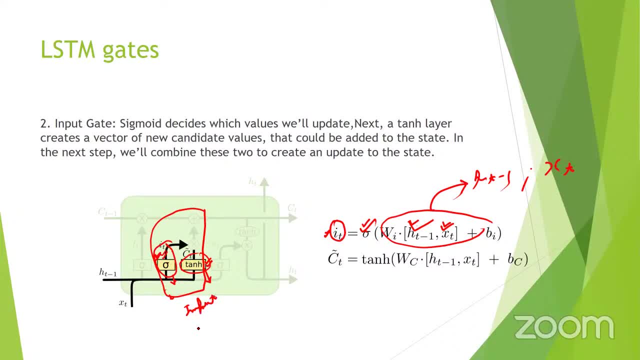 input gate. right, we are inputting, we are giving some information to it, so in this input gate will filter out the information that help. that will help it to kind of get a good function between your white t plus one and your previous phase data and it will reject all the. 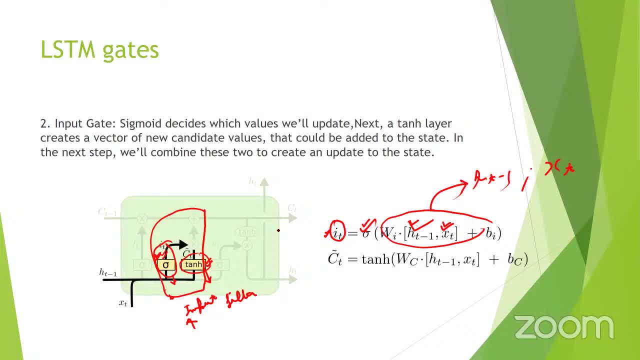 information that is not helpful for it. right, that's why this sigmoid layer came into picture. so that's why this sigmoid layer came into picture. now you know that, okay, this sigmoid, and you decided that- what to take input and what to take output. now, what is the role? 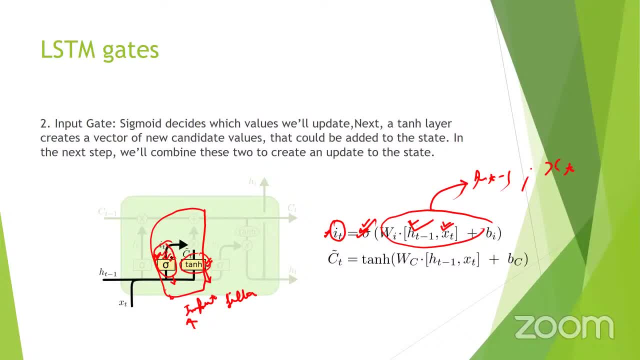 of this tanh then? right, so this sigmoid just told you that, okay, this particular thing you need to take input and this particular thing you need to take as output, but you have to pass that information to yourself. right, so that information will be passed by performing the tanh activation on the. again, this: 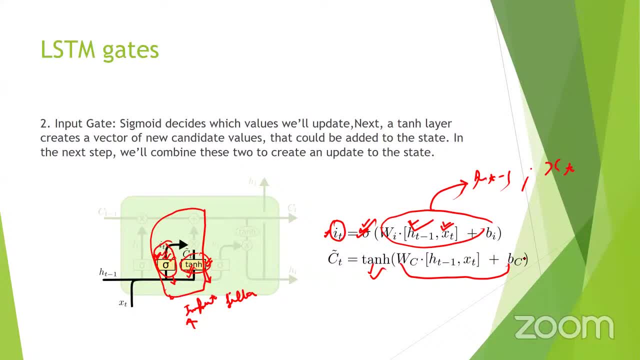 particular equation. here your weights and biases again will be taken to the output different. so what exactly this tanh or this particular tanh cell here is doing? it is doing two things. first, it is extracting my future. it is doing my future extraction from current input, from current input, let's say from xt. so 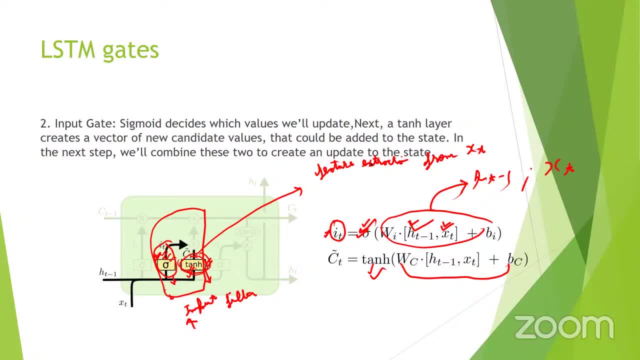 it has extracted some of the feature that are that are important to learn, or you can just say, extracted the future from your inputs itself and code it back particular thing so that your output is extracted. as you can see here, my input is extracted from current input so that your input is. 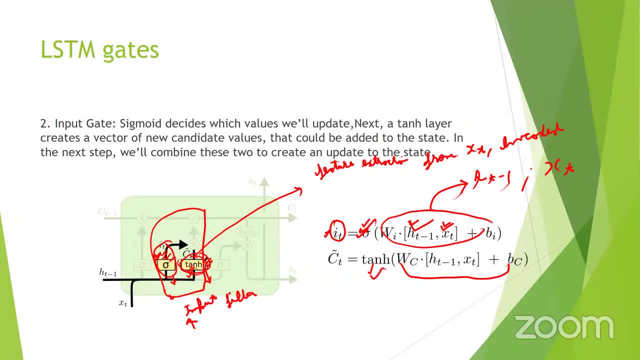 your neural network or your machine can understand. So this 10H is handling that particular thing. It is extracting features from all the inputs and encoding them. And this IT, for this IT, this complete thing, is your CD. that is your feature, extracted and then coded. 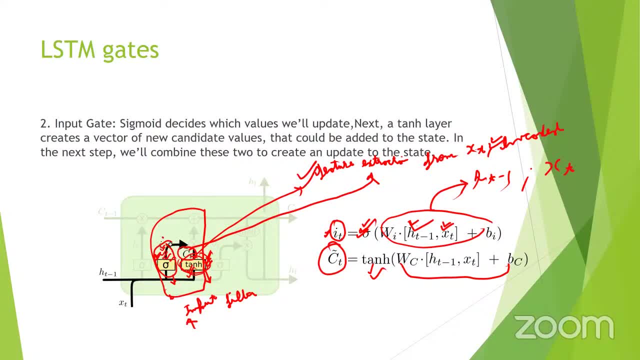 for this particular part And this IT. it will make the decision that from these extracted feature which one to take and which one to forget. right And again, if you see, at this particular point, wise operation, multiplication is happening. Obviously multiplication will happen. IT into CD. 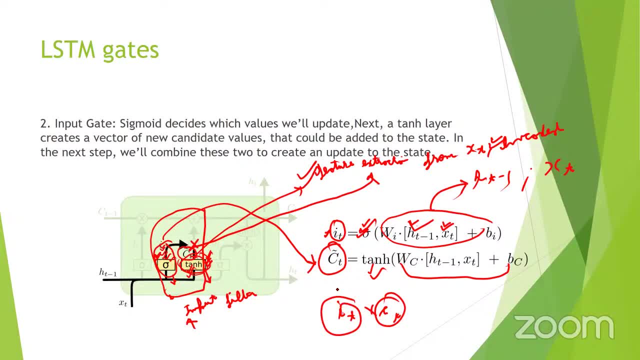 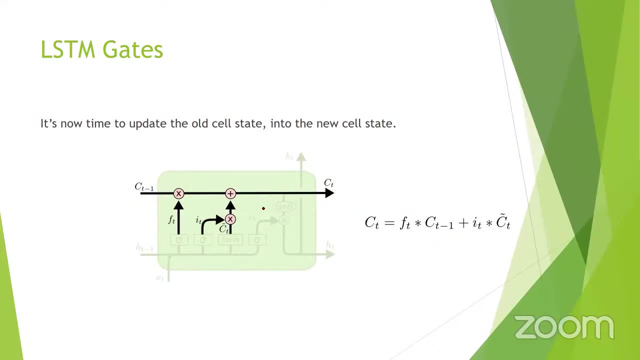 So these are your extracted feature And these are your. you can say your decision of a sigmoid layer, which one to take, which input to take and which one to reject. In this way your input gate will work right And if you see the particular output here. 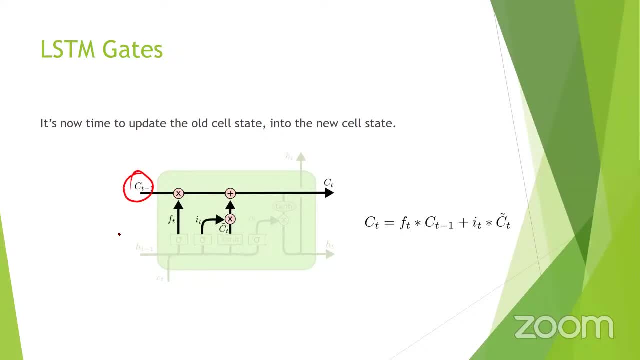 Now coming back to your cell state itself. right Now it's the time to update the old cell state into the new cell state. So from the previous cell I got my cell state CD minus one Here from the forget gate I got some information. 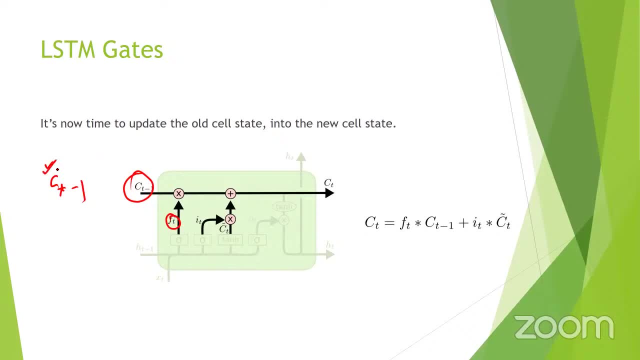 which information from the previous cell state to take and which one to reject. So I multiplied the CD minus one with my FT CD minus one And now from this input gate I got the information for the new inputs or for the inputs for the current time. step T: 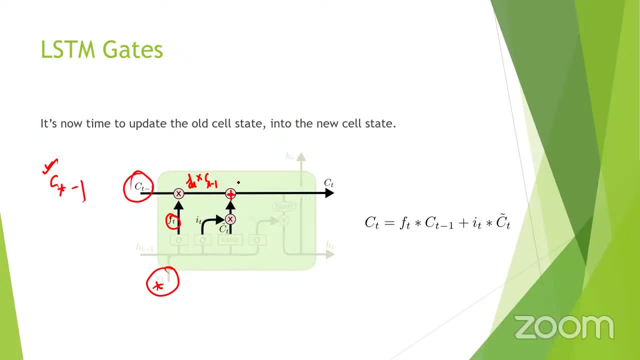 And I will be adding those information in my previous cell state. So here it will come: FT into CD minus one, plus IT into C dash T, where C dash D is your output from this candidate layer And IT is from output from the sigmoid of your input layer. 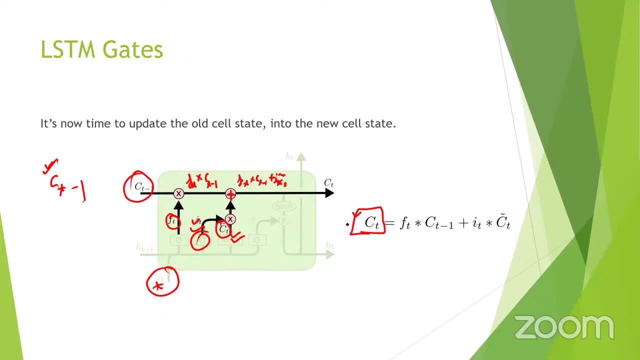 So if you see your new cell state will be equal to FT CD minus one, plus IT into C dash T. So if you see your new cell state will be equal to FT CD minus one, plus IT into C dash T, So your new cell state is having the information. 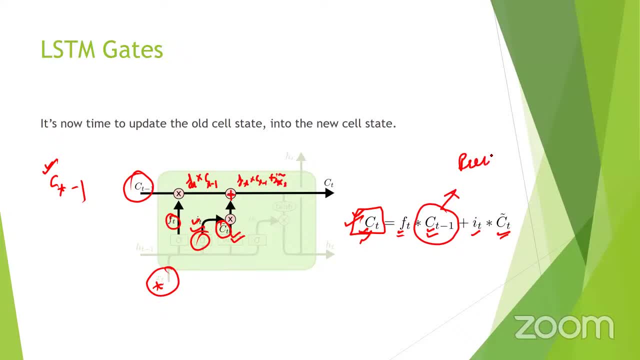 some of the information from previous cell state, previous cell state. but you can say information, or you can say data encoded from previous time steps, right From previous time steps. This particular thing is representing that. or you can say this is representing the time dimension. 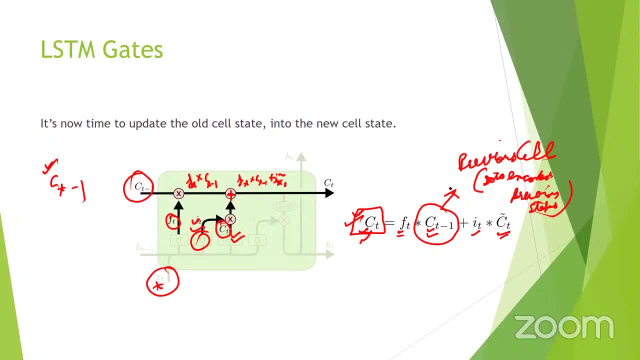 inside your learning. So this is the learning of LSTU, right? So we have information from our previous time steps itself And in that particular thing, we are adding the information from my current time step, adding this candidature CD dash multiplied by IT. 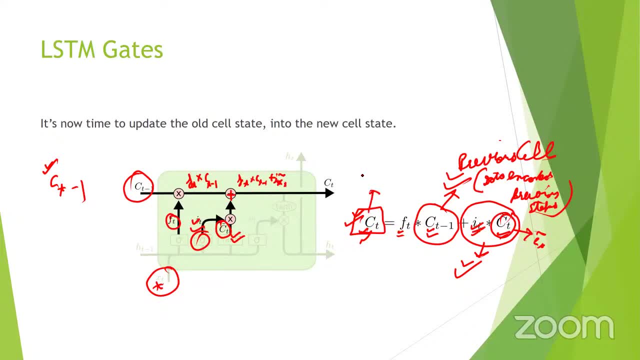 So now this cell state has been updated, updated to the information, having previous state information as well as current time, Right, So these are the, you can say updation of your self state. Now, from this particular LSTM itself, we have to give some output also. 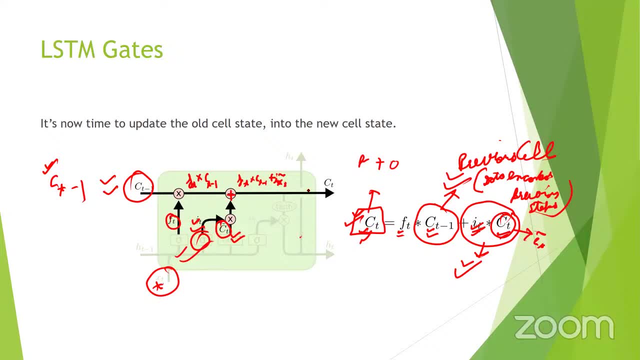 This cell state is directly going here. if you see, this cell state is directly going to the next cell and let's assume that it is connected to the next time step. that is my white E plus one. I'm also- let's assume that I'm also considering this white E plus one. 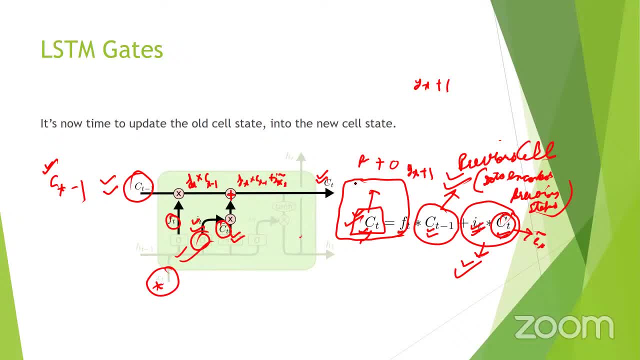 in the relationship for getting some y value right. so again, in that y, t plus one, same operations will happen. that information for that t plus one cell step will be stored in the similar way as it has done for this particular time step. now your cell state is sorted, now how to handle your. 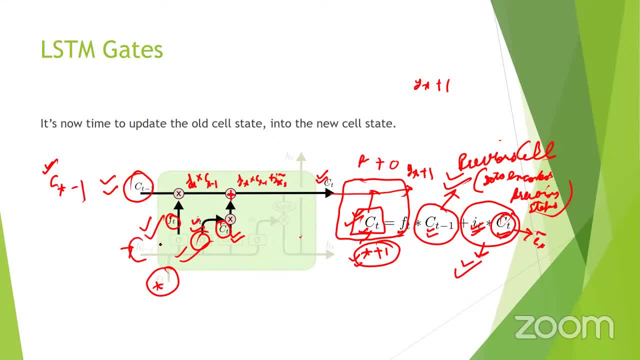 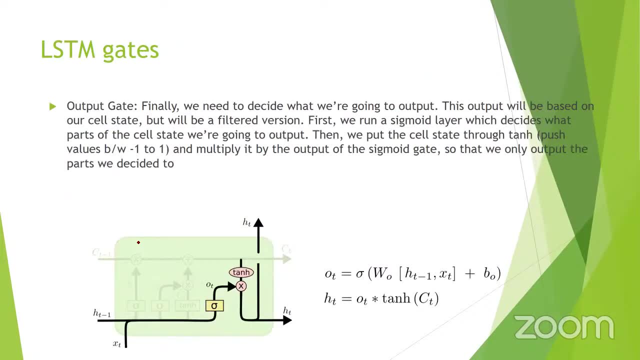 hidden state, the hidden state that i was getting from my previous step. right and in the beginning, as i said, your hidden state and cell state are kind of interrelated with each other. only so, for that particular thing, your output gate comes into picture, giving the output to your next. 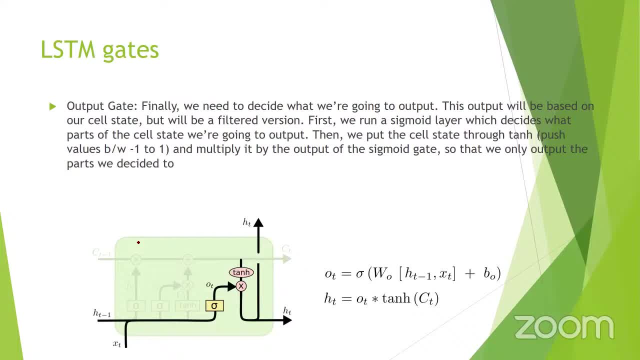 uh, your next cell, uh, your next time step. so basically, this output is nothing but your cell state. but in the filtered version itself, right in cell state, the cell state was having the complete information of previous data points. and i said that your hidden state will have more information about the current, uh, current cell itself, right. so again similar type of 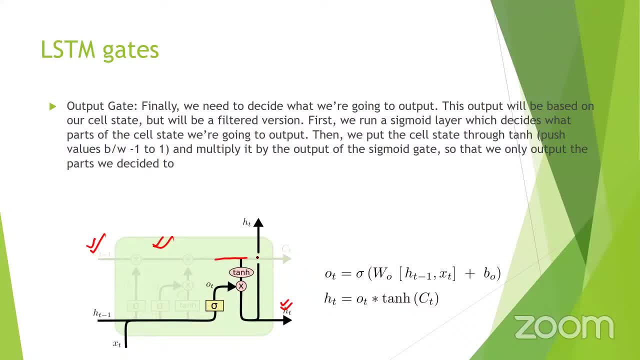 thing will happen here. if you see, this cell state is coming here. this is my one cell state and this is the same branch from that cell state itself. now this cell state will be passed. the cell state will be passed through 10, this particular 10 h and one other, uh, this: 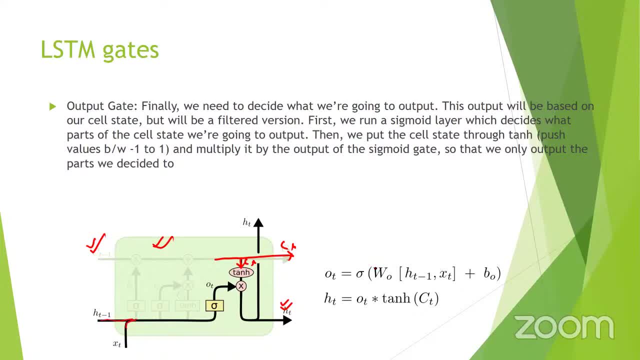 hidden state from previous layer and xt from previous layer will be taken and output for from that particular sigmoid cell will be this ot and now this again ot will decide how much of your this current cell state you want to take inside your ht current hidden state, right? so this ot again. if i tell this that, if this ot is again considering the 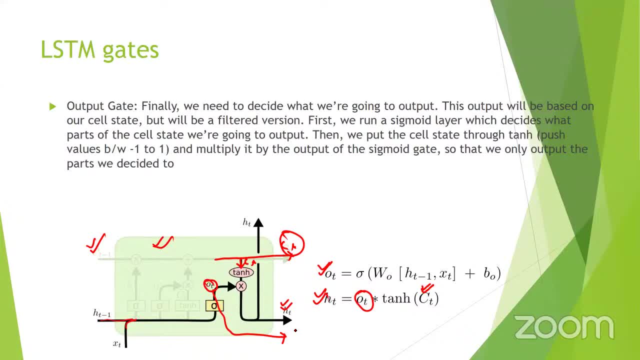 information. how much to remember, how much to forget? so this particular thing is that, and this ht here, uh, dot ht, this complete ht, the hidden state will be calculated by multiplying this ot with the 10 h of my current cell state, and this particular thing will give me my hidden state. so your, you can see. 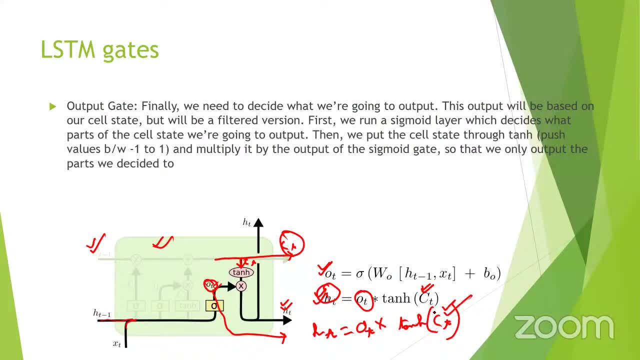 your hidden state is kind of related with your cell state itself again, depending on how much to remember from the current cell state and how much to forget and taken, uh, taking this 10 h even so, if we show in and so on the complete lstm in high level when we are talking about sigmoid. 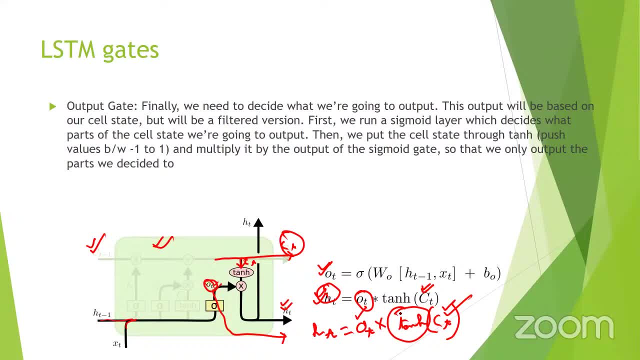 with when we are either amplifying the things or diminishing the things. when my sigmoid layer output is nearer to zero, i am diminishing that particular thing and whenever, whenever it is nearer to a one time amplifier, i am completely using it and your time- 10 h- is basically used for normalizing. 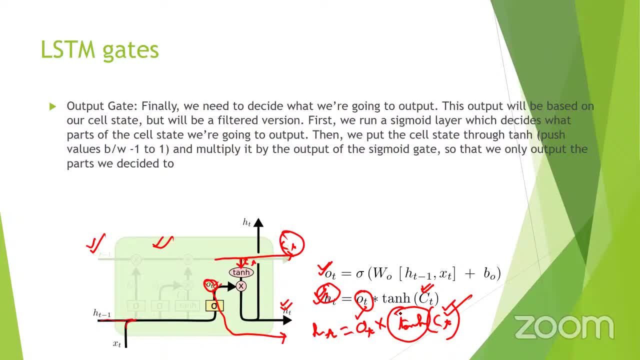 for making the normalized encoded of your data normalized encoding of your data, right. so in this way we are able to calculate the hidden state of uh, this particular cell, and all these things again will go on. are we going to see a python implementation phone? yes, permit you're. 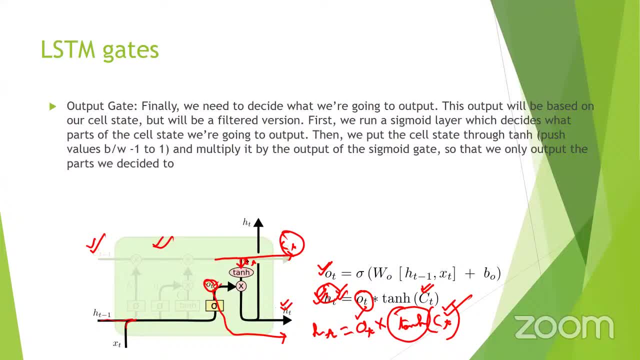 going to see that. but yeah, this is the addition behind your lstm cell. in this way, your uh again and all other things, whatever the things that takes place for the training or simple n, and all the things go on in the same manner itself. there will be your gradient descent, there will be. 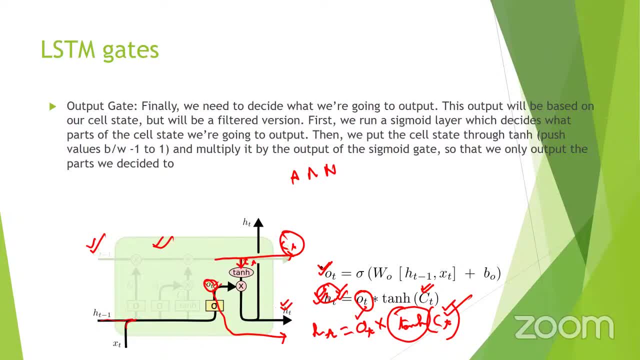 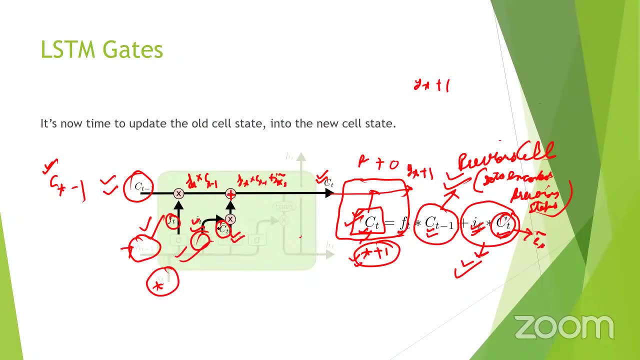 different, different epochs, your forward pass and backward pass, all things will be there. but if you remember, in a- and we just learned one w and c for one cell and here, if you see your lstm cell, your one w and b is present. for your output gate itself, one w and b is present for your input gate, one w. 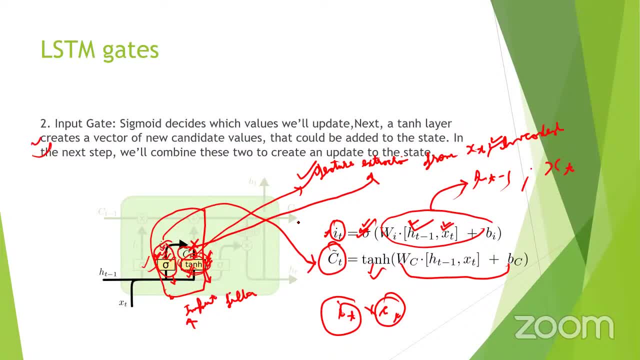 and b is present for your uh, this forget gate, one in uh. one w and b is present for your this it here- and one w and b for this city. so multiple w and bs are there. basically four w and bs will be there. if you see, here let me show you one w and b. 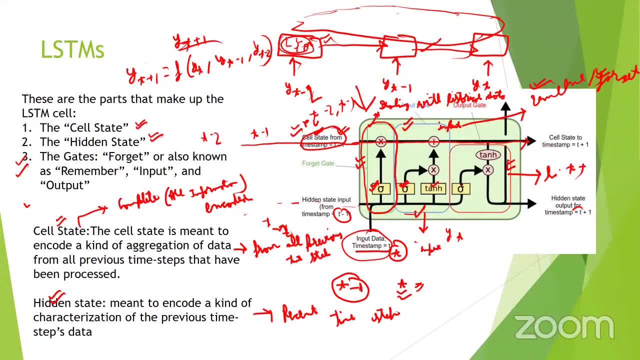 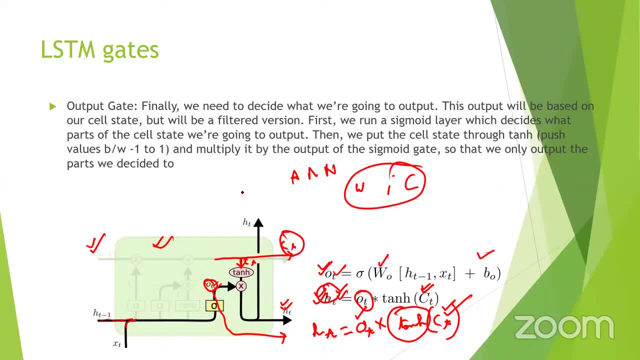 for this single thing, one for this one, one for this 10h one and one for this single one. so your a and then we are just learning one set of w and c. but for your lstm we are learning four sets of w and c. that's why these are computationally heavy, also for training. 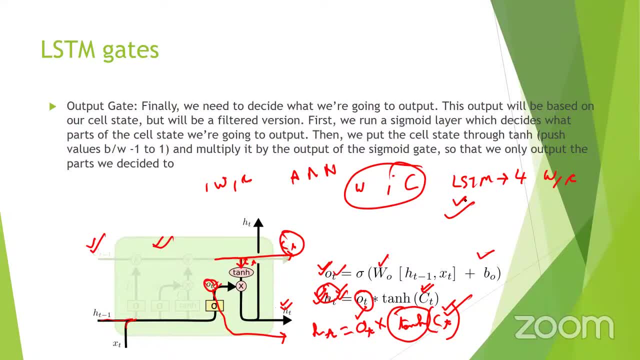 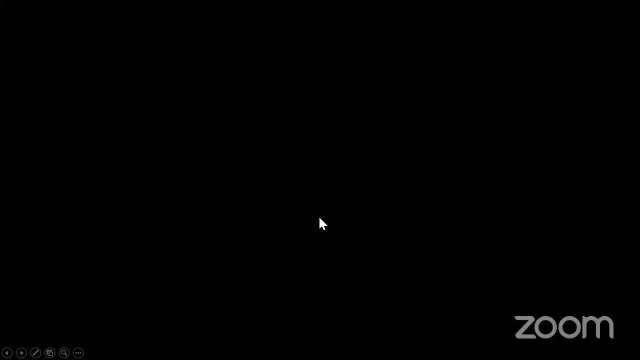 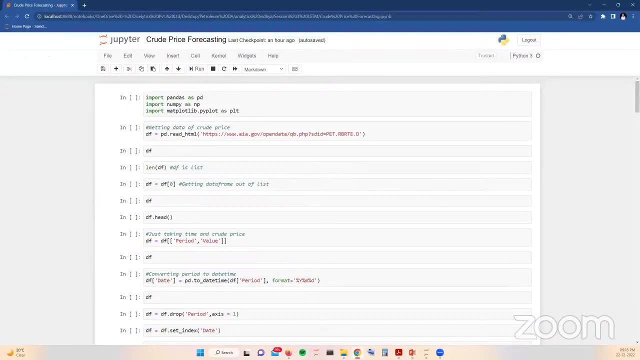 uh, at lstm cell, and then i hope, the intuition behind the lstms are clear. so let's jump on to your power coding part. if you have any doubts, you can ask in the chat box. yeah, i will be sharing the as well as i will also sharing the code, and you can also find the complete code and presentation. 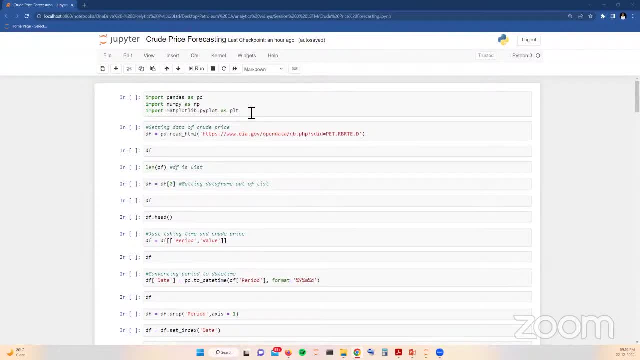 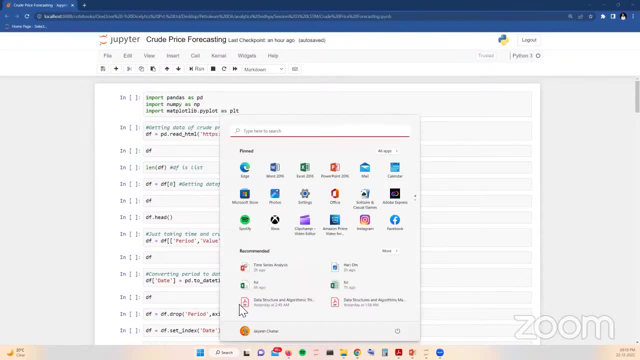 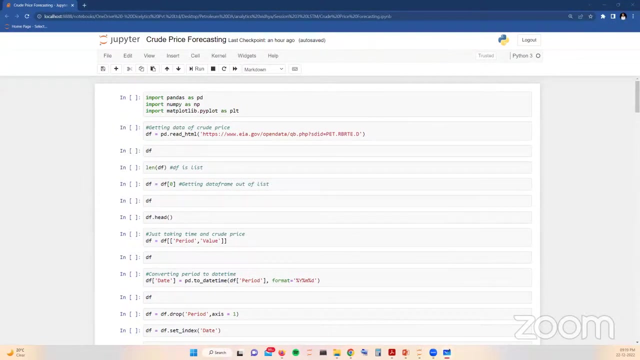 on my github profile. also, at the last i will also share it. but yeah, let's start with the coding itself. and uh, give me a second. before going on to coding, let me tell you one more thing: how exactly the data will be prepared for passing it inside your lstm network, so that it will be easy for you guys. 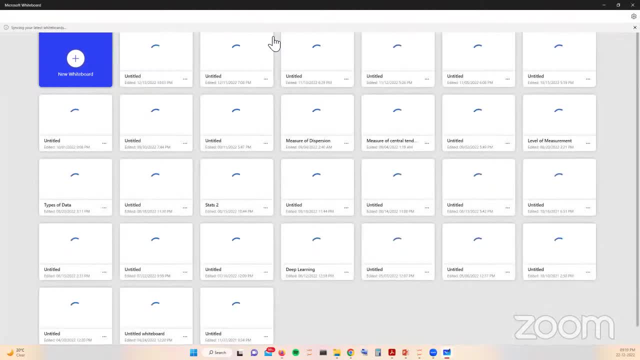 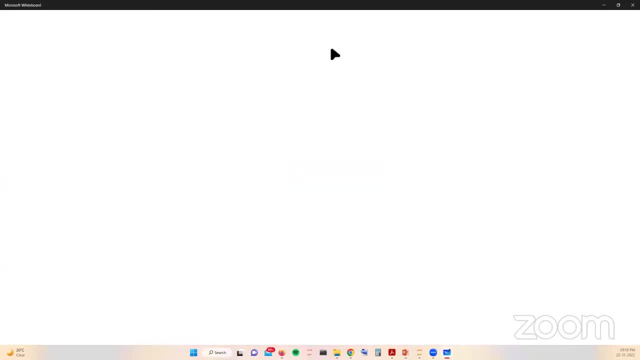 to understand. okay, so here i'm talking about rand and machine mail. also let's combine rand machine and machine gas. but basically it consists of data from several, several sensors. sensors, data right, and my problem statement is牌. data object is to determine that, whether anomaly, or whether my machine broke down or not. so my problem 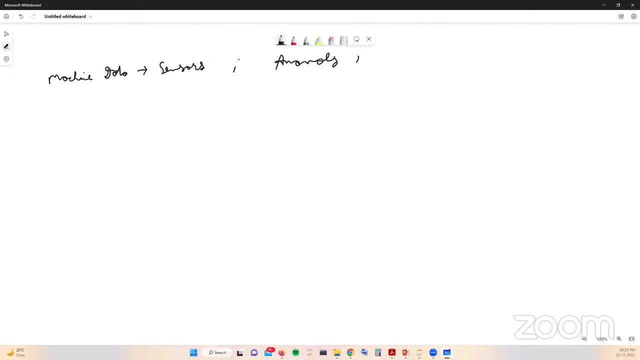 statement is anomaly detection, right? so i am just taking that i am having x1, x2 and x3, these three sensor data ports. let it be pressure, temperature or whatever right, these three features are present. my target value or target variable is y, that is, whether anomaly is present. 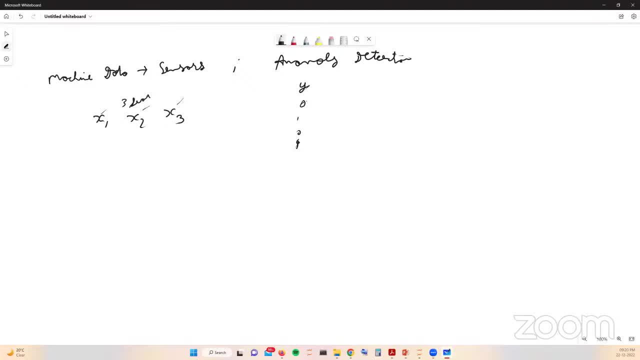 or not. so it will be 0, 1, 0, 1, right. 0 representing normal condition, 1 representing my anomaly condition. right now, i know i am having this uh data from my sensors. these are time series data, right? so basically, this anomaly, that whether anomaly is there or not, it will depend on the 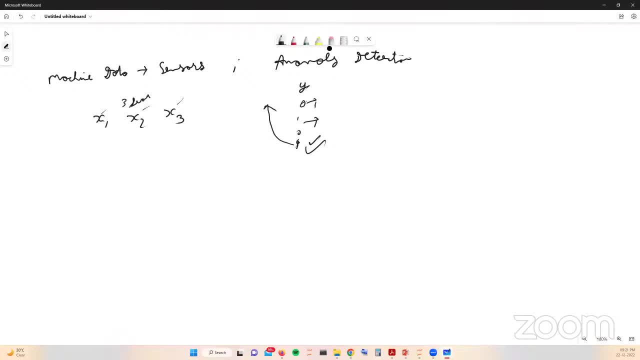 previous data, data points itself, previous behaviors of my uh, these sensors for data itself, right, and now let's assume that i am having how much? let's say thousand rows of data right for my x and y's. now how will i feed these x and y's inside my lstm architecture? 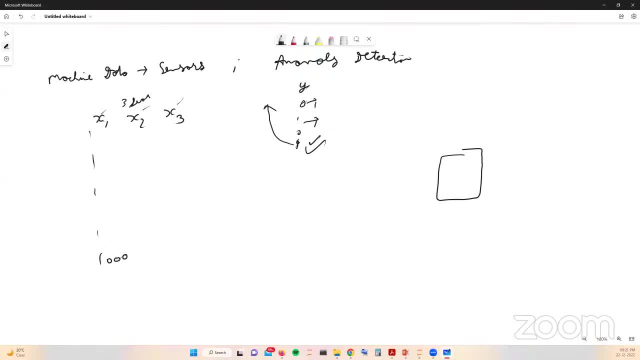 right. basically, if you know your aiml model is nothing, you input x here and you also input y here and you will get a fx file, fx right. basically a function that is mapping your y with respect to your x. now, how to and whenever we are talking about? 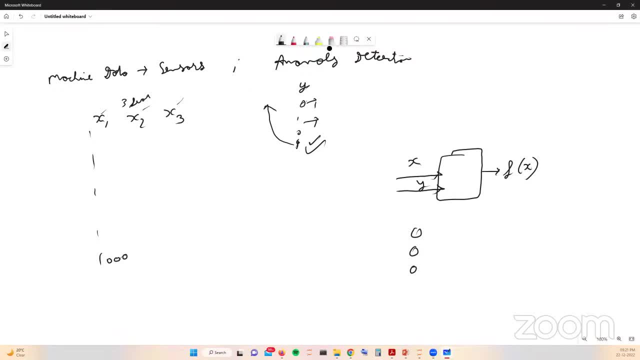 simple: anns anns your artificial neural networks. we just give inputs of your x1, x2 and x3, and there is some, let's say, neural network here here and it is directly mapped to your wife. in this way we generally give inputs, but the same thing is not true for your lsdms. 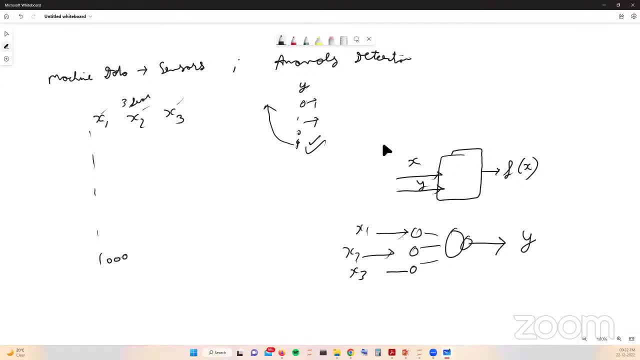 so in lsdms, first of all, you have to make the batch depending on one particular time window. right now, this time window, you can decide by your domain knowledge. for example, here i'm talking about the machine that i am talking about, the compressor data. so now, if i am having a great mechanical engineer with me, he will. 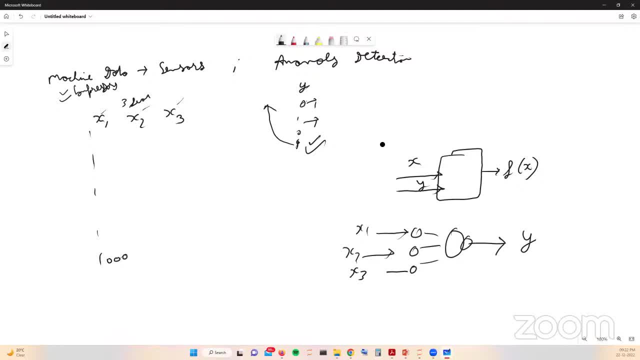 definitely tell me that. okay, your compressor data or your breakdown of your compressor is kind of dependent on your last 100 time steps data, or let's say i am getting these data per second, so he will tell me that. okay, your, if whether there is anomaly or not for 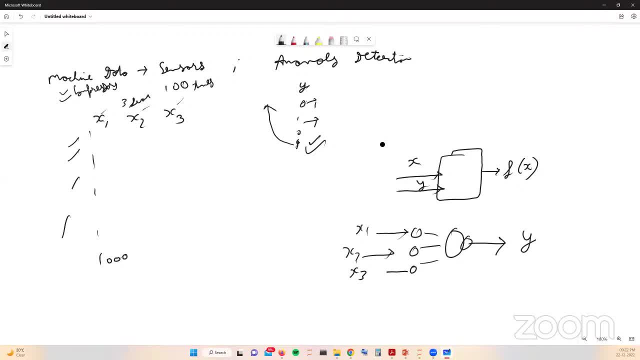 a given machine or data in a given machine. it is dependent on your last 100 time steps or the last 100 seconds. so what i will do here, what i will do here, i will take my first 100 data points, starting from my x1 and if this is my x1, x2 and x3, these 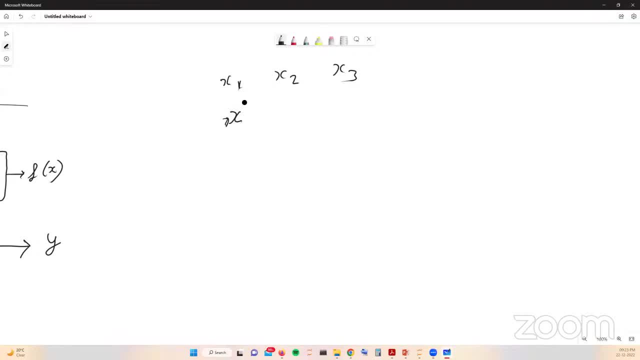 features. right, i will take my first 100 datas. this is my x1, 1, x2, 1, x3, x4, x5, x6, x7, x8, x9, x10, the similar way. this is my first time step data and this is my 100th, 100th time step. 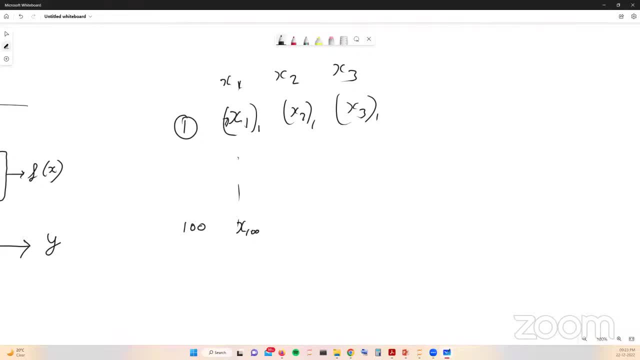 data. that is my x100. it is x100, x, 200 and x300. i will take this complete batch, this complete batch of data, and i will try to map this particular data with my x200, my y 101, right? so i am just telling that i am operating my machine for 100 time steps and my 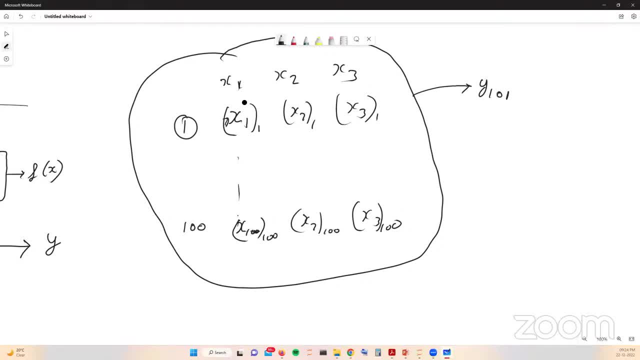 y 100 for my machine condition at 100 month. second is, depending dependent on these previous 100 time steps data right, these previous 100 time steps data. so in this way, if i am, if my neural network is signing, finding some of the different nature of these data points for these 100 steps, 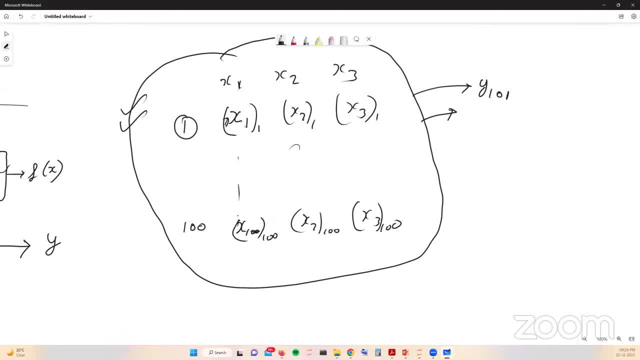 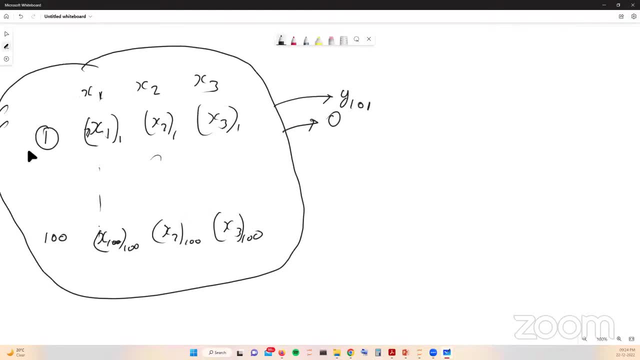 it will automatically tell me that. okay, for 101. today, your, you will face an anomaly. now i have to create my uh, this particular uh- style of data, right, i have to create the data inside my lsdm cells in this particular style itself. so, how i will uh, how i will do it right? 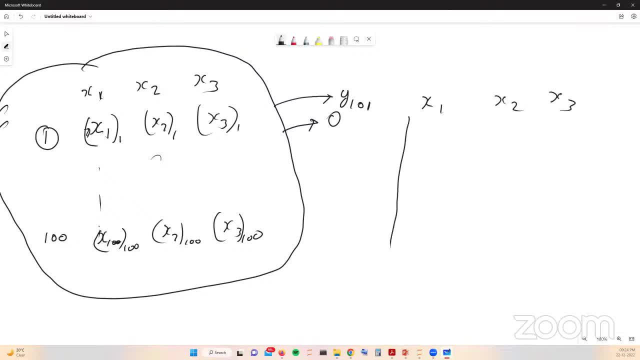 x1 right. and i said that my 101th day condition, my 101 30 condition, is dependent on first 100 days right. in a similar way, my 102nd day condition will be dependent on last 100 days, again, 2 to 101. my 103rd day y will be dependent on. 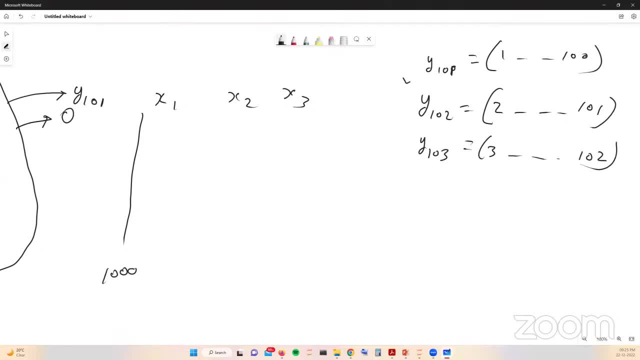 on last 100 days, again, right, so i have to make my batches in this way. so what i will do this is thousands, right, so i will take x1, x2, x3. i will take first 100 days data. i will make a one batch of it, right, and this particular thing i will map with my y 101. now my next batch of data. 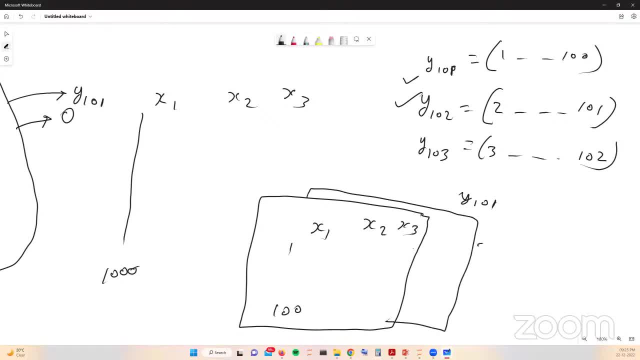 this particular thing will start from second day and go till 100, one day right. in a similar way, my next batch will start from three and will go on this 102. this one will be mapped with y 101. this one will be mapped with y 102 and this one will be mapped with y 103, and this way. 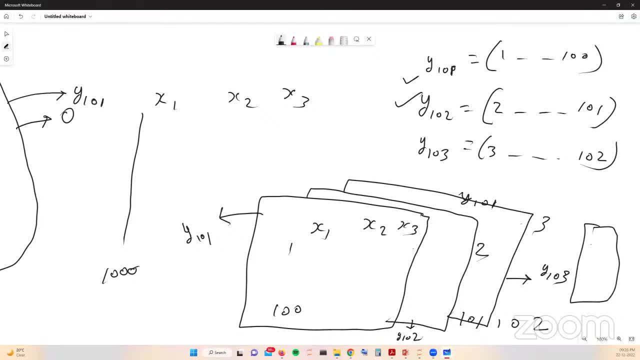 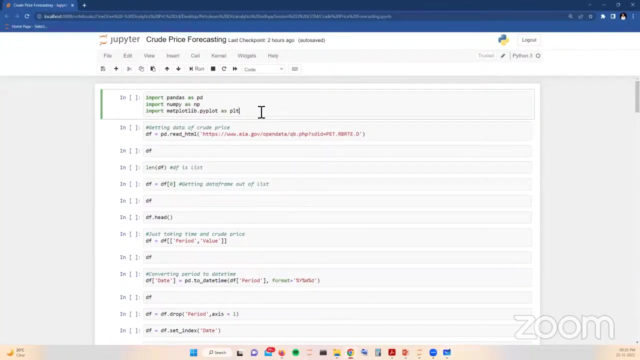 this complete x and y will be passed through my lstm architecture. you and it will be able to get the relationship of my y 100 plus t with my previous learning step. right now let's jump on to the coding and see how to create this particular data things right and for this particular hands-on coding. first of all, i am 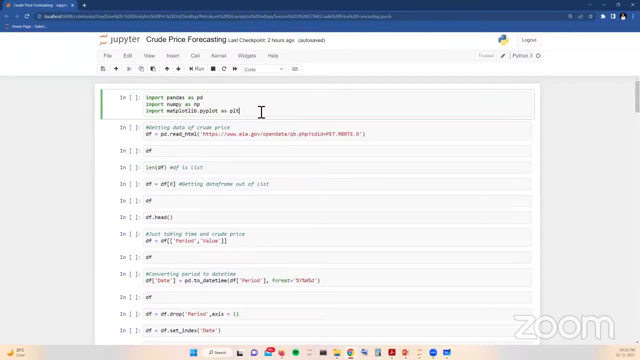 taking the example of univariate time series forecasting, and i'm taking as i am a petroleum engineer and i'm taking as i am a petroleum engineer and i'm taking as i am a petroleum engineer from my bachelor. so from my education point of view, education background, i'm taking account, i am. 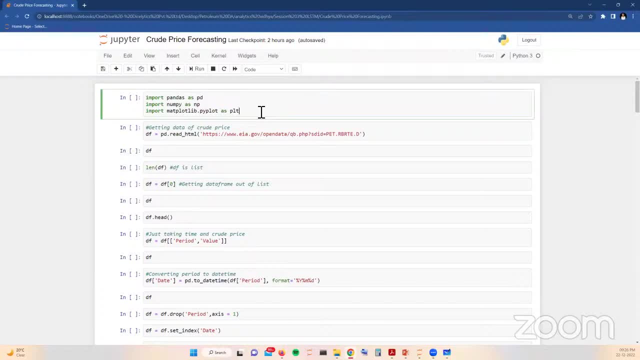 taking the project of crude oil price for puzzle right and in a similar way you can also forecast some of the shares. but for practice purposes only. if you are going to make decisions depending on this particular lstm models, then if you go into losscom just for practicing lstm, you can kind of 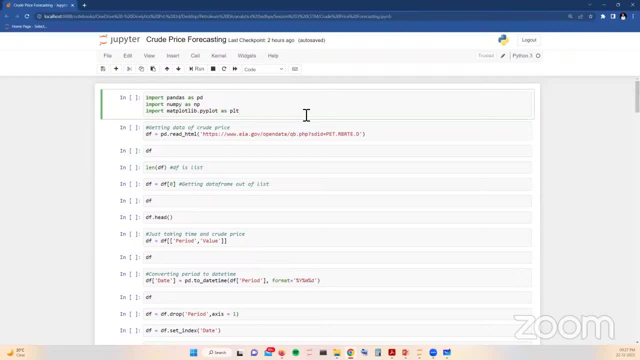 pick up this type of purpose, just for practicing lstm, you can kind of pick up this type of purpose, but again, how we exactly are not able to do these things. again, the limitation part we will discuss in the end of this video. so first of all, i am importing all the libraries that i have. 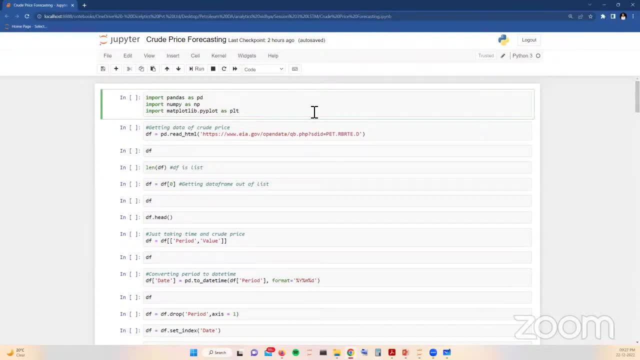 going to use- i am importing my pandas gumpy and for plotting petroglyph- right- these are imported- and for getting the data of my crude oil price. i am using this particular website where my brand crude price data is updated every day, so i will be using that. 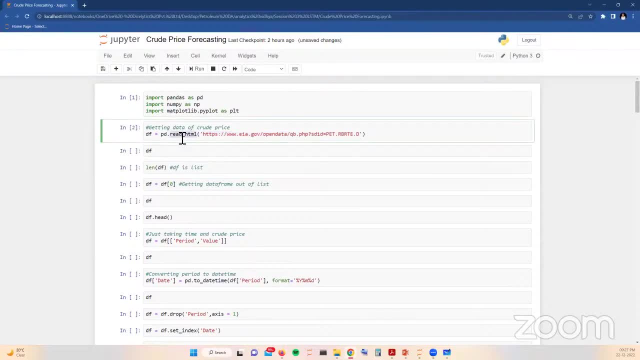 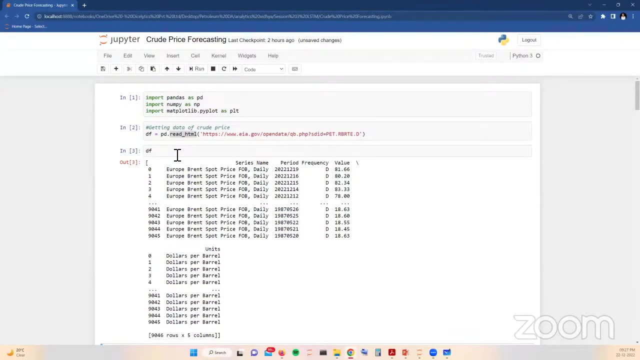 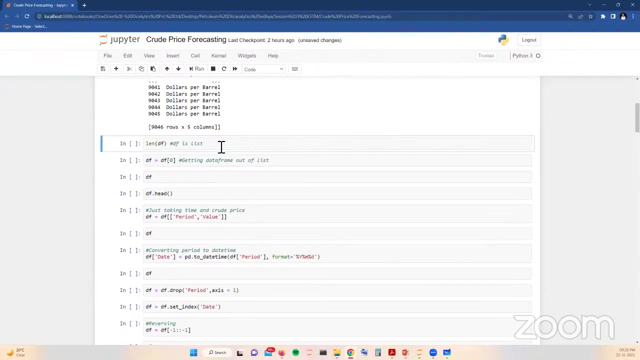 particular data- and i'm just using my read html function of my partners, right? so this is my data frame, if you see it here, and as i have used v-tml, my complete data will be stored inside a list. so, first of all, let's get this particular thing in the data frame itself. so by indexing the first element, 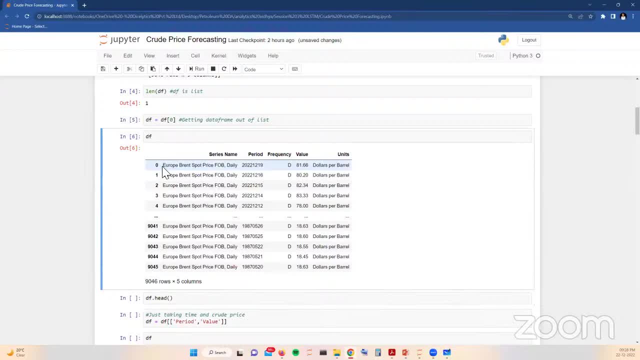 i'm going to be using the data frame itself. so by indexing the first element, i'm going to be indexing the first element, i'm going to be indexing the first element, i'm going to be got my data. so here you can say: uh see, this is my, you know, brand crew. basically, there are different. 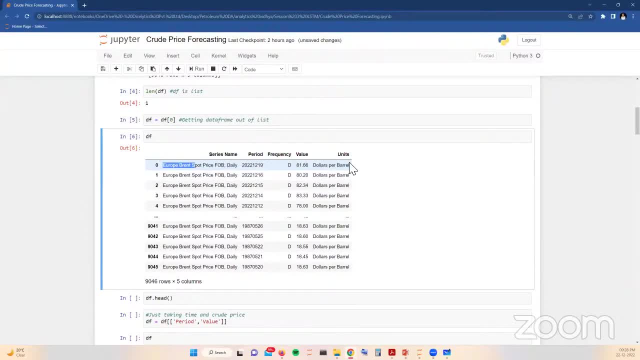 different types of fruit again. you will not know. indeed, but yeah, this is the data points for my brand crew here. uh, it's mentioning brand crude. this is my basically time step. it is representing that. okay, the data is for 19th december 2022. frequency is my days per day. data has been taken. 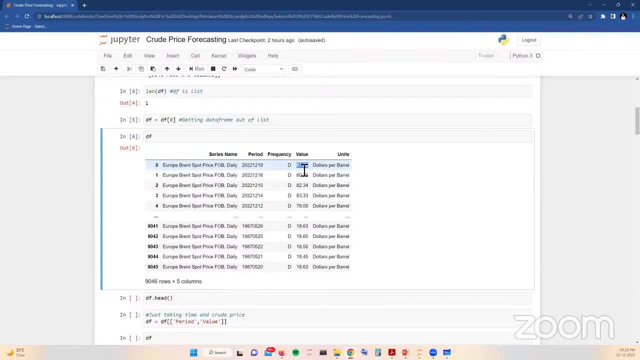 about and what was the value or what was the price of my brand crude of one barrel of oil on that particular day. so it was around 81 dollars. but let's, uh, let's get rid of these crap things that i don't use, uh, that i don't want, i just want. 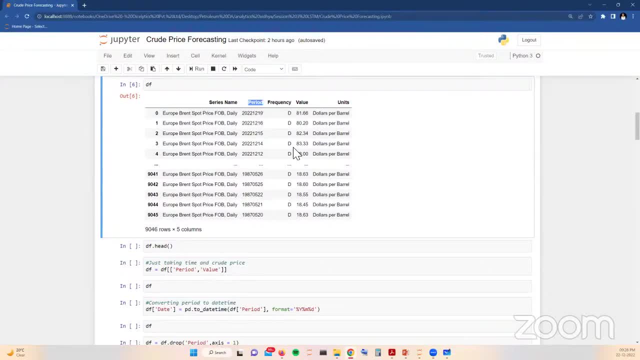 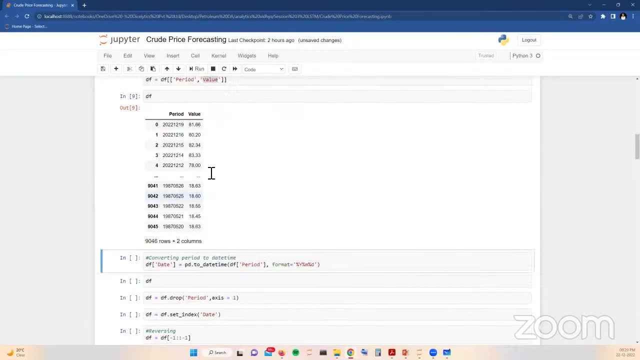 this value thing and i just want my uh date right. so first of all, i'm getting these things out of my data frame period and value. so this is my final data frame. first of all, let's convert this period into date time format again also. so i'm using my pandas function, which 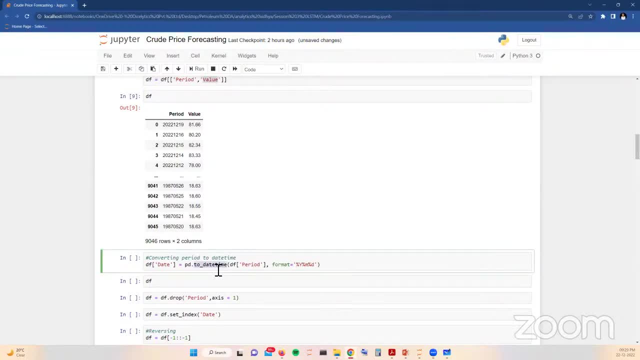 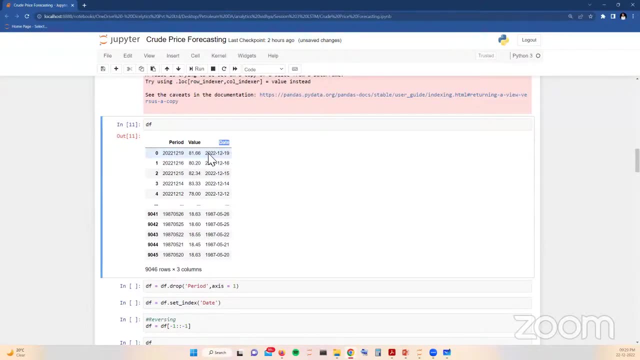 is used to get time for converting this period into daytime format. right now, if you see, here my period has been converted to date time here- 1912, 2022, and i am having the data from 20th by 1987. right, a lot of data is here i'm going to use. right, this period is not necessary. 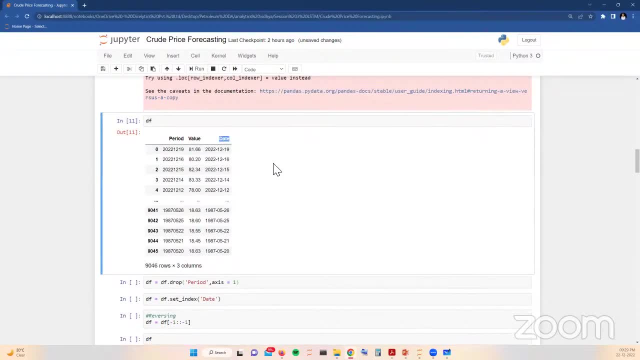 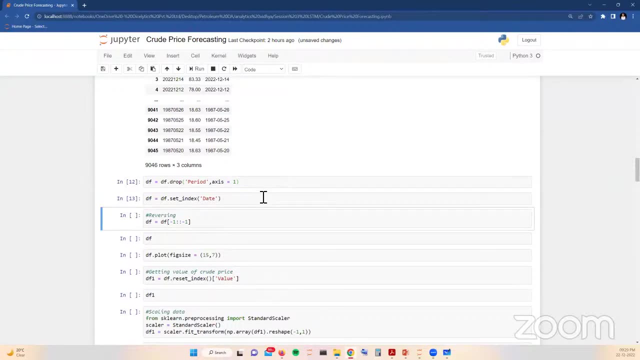 now because i have time information from this date column itself, so i'm going to drop it. setting the index as date: these are some of the basic points, so i'm not going into detail, right, just preparing my data frames. so my data frame: here i just reverse the data, so i just want the past data first. 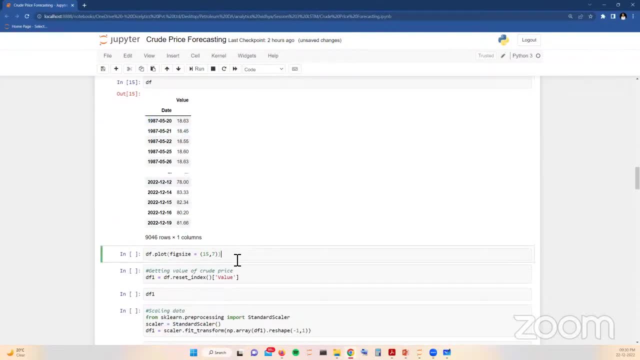 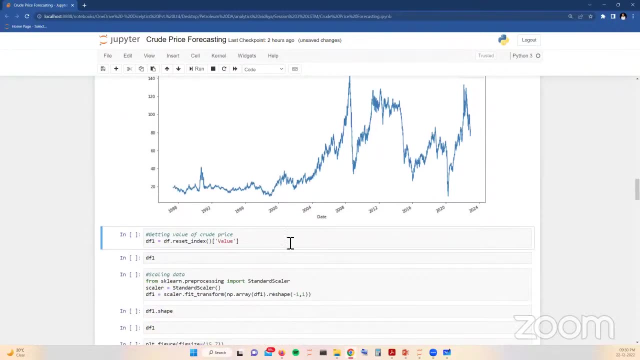 so i just reverse the data itself, nothing else. now, first of all, let's note: so this is my time series and it's looking like right now let's just get the value of crude only. so i'm storing this particular series inside this variable df1 here. 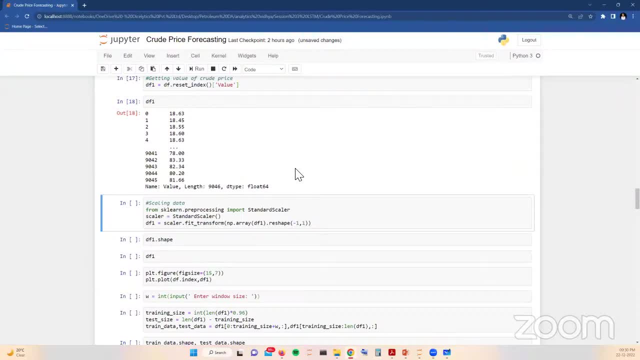 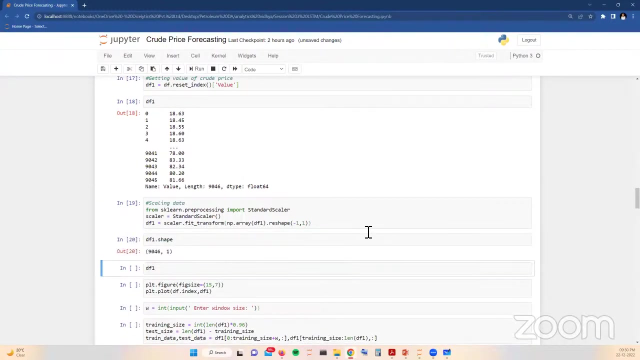 back route values. only now we will be scaling the data because our neural networks are very sensitive. scales right. so i'm using a standard scalar here for scaling my particular data, just using sk learn for scaling the data and after that just storing that particular thing again. so this is my scale version of the data. 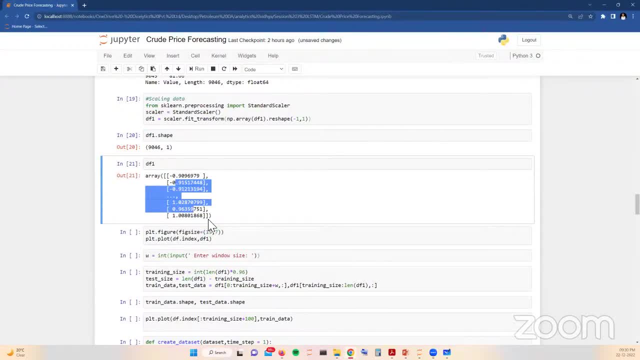 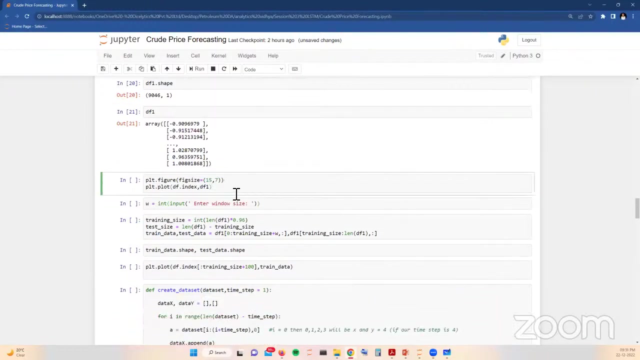 and i will be sharing the notebook and i will be sharing the link of a github also where you will get the load directly and also the analytics with. the guys will also share it all, share it to you all there, but for now just focus on the possibilities right and now. if i see this scale, 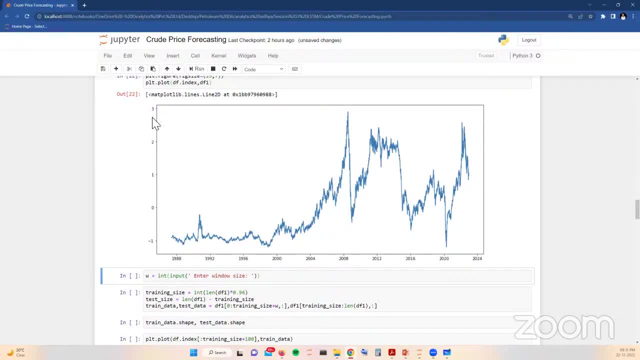 data. this one is my scale data. you can see on my y-axis my scale has reduced to minus one, two, three, right, and here this was the original data scale of the data, so i can now see the data. i want to take this into my organization and i can see that while i'm doing this, i can see that you can see the whole data. 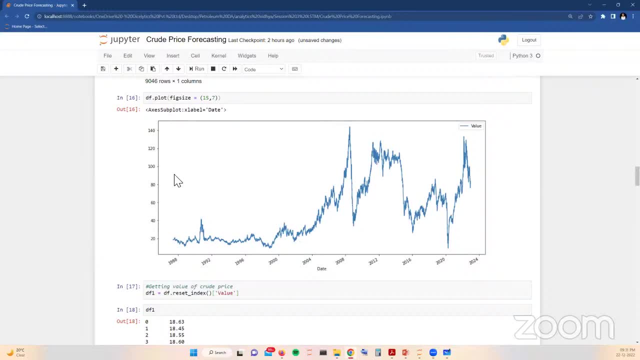 and i can see that right, and if i want to look at the data's in between, this is going to be my nodes and i am going to go in there, so then the data is going to be shared with you, all right. so, for example, this was the original data, so i just scaled using my standard scanner. only nothing fancy. 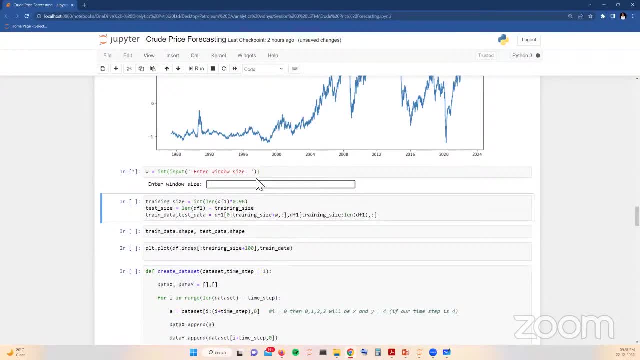 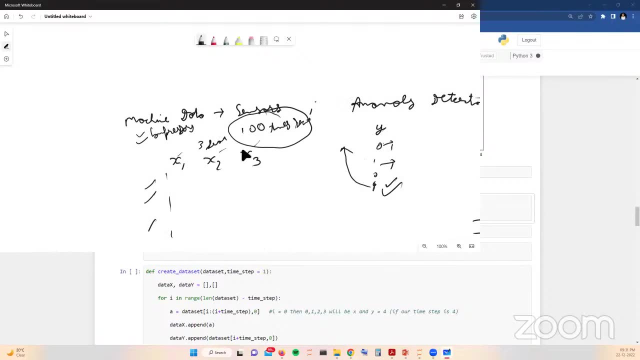 right now i am taking the window size, the window size that i discussed here, that this particular window size, this time step size, here for my machine data it was 100 time steps, right given by your again domain exploit that particular thing. i'm giving us input here. so here again, 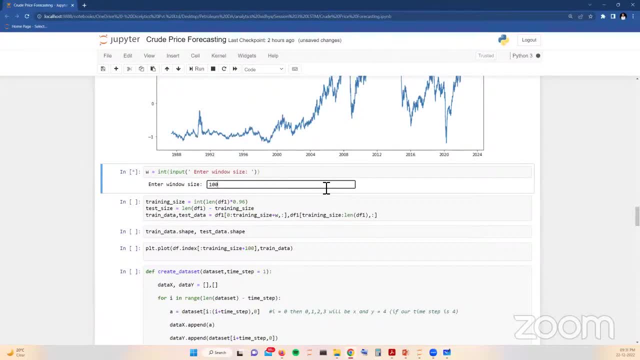 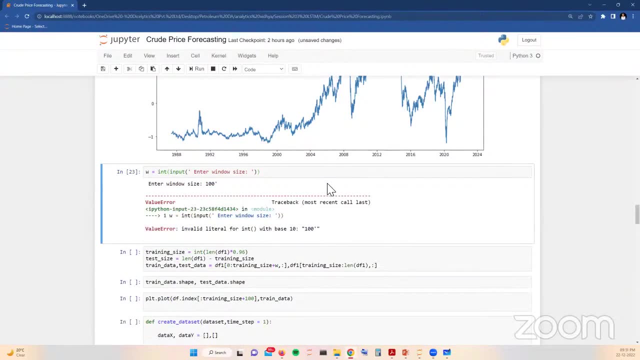 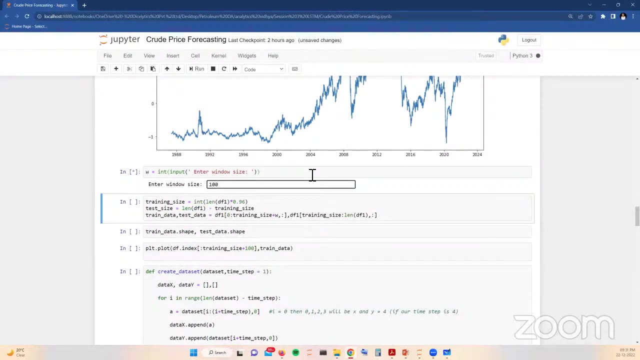 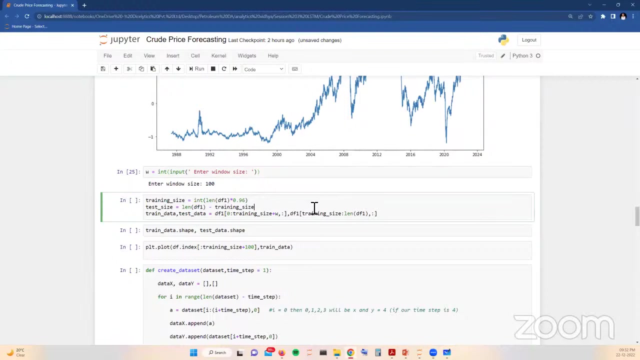 i'm giving, let's say, 100 days data. i'm just mentioning that my 100 first day of crude price is dependent on the last 100 days of crude price. okay, i've given, given the input, 100. now i'm just splitting my data into training set and test set, and 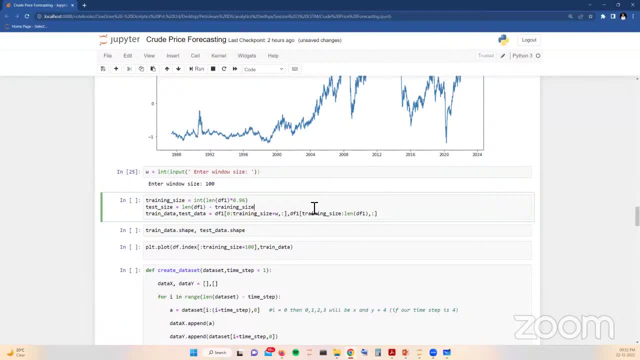 as you guys know, we are talking about time series data. okay, okay. so if there will be sequential split by default, if you use train test split from sql that randomly splits your data, that is not valid for your time series data. so you have to sequentially split your data point or complete data itself. so that particular thing i'm just moving here. 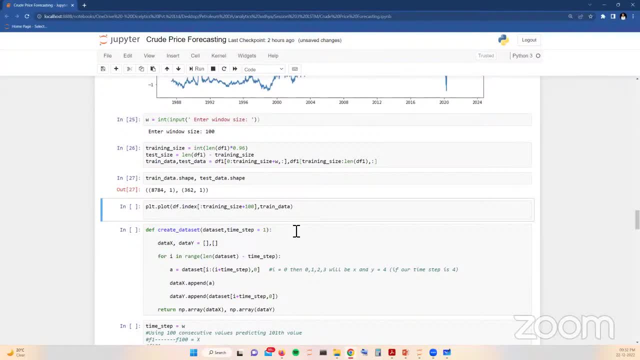 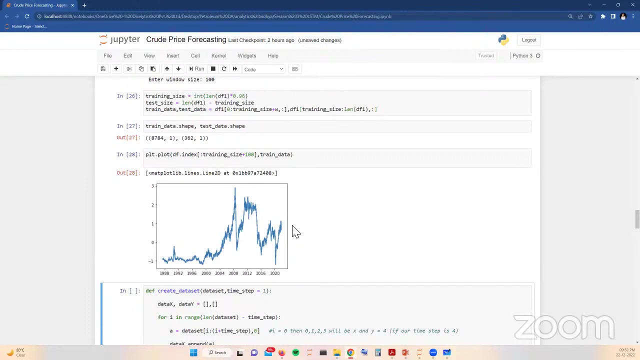 so this is my shape of my training data and testing data, having one feature that is my price itself. that is feature and that is target value also. now, this will be my complete training data. do you have a good mathematical explanation paper? how lsd? yeah, i will share you the. 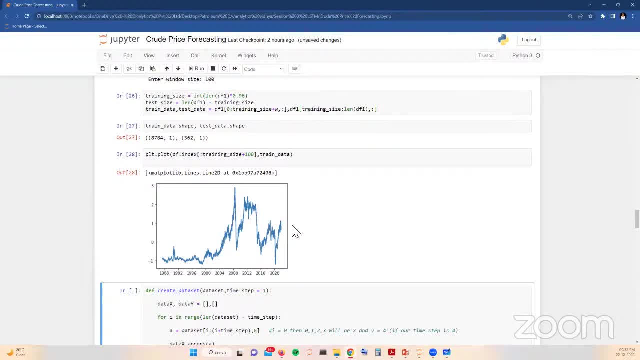 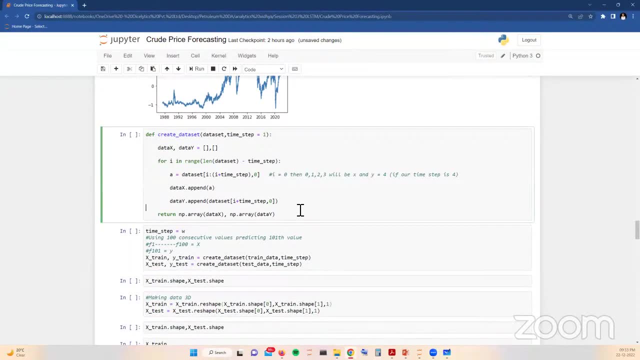 original paper of lsd, itself the original research paper. then they came up with the lstm and how they moved on from rl Embedded儿 and to LSTM. Right now, this particular function, that is, my create data set function, that is taking care of the the creation of my batches, depending on my window size. so if you see the logic here written, 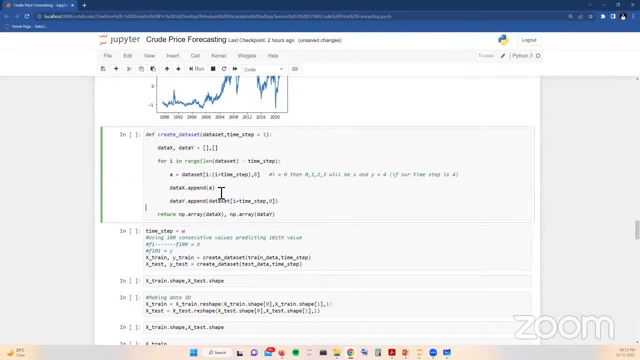 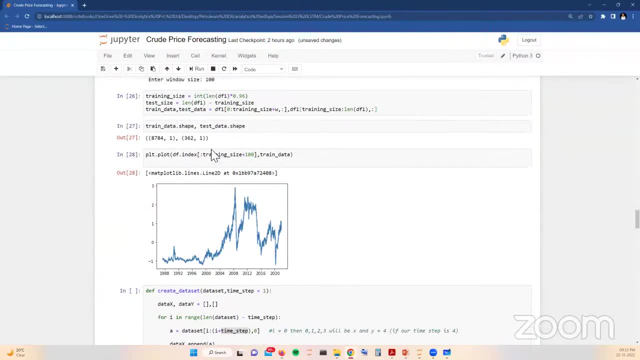 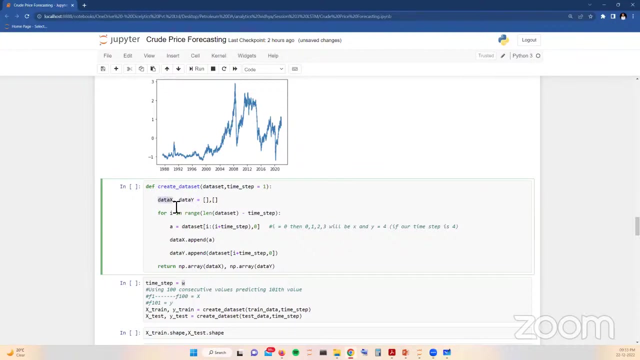 in my for loop. what I am doing exactly here is I am taking some my time step. that will be my window that I have already mentioned 100, right? so I am just taking my data x and data y. in my data x I will be filling up first 100 days of data and in my data y I will be 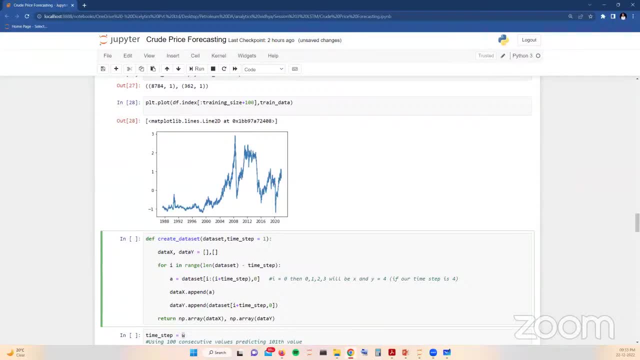 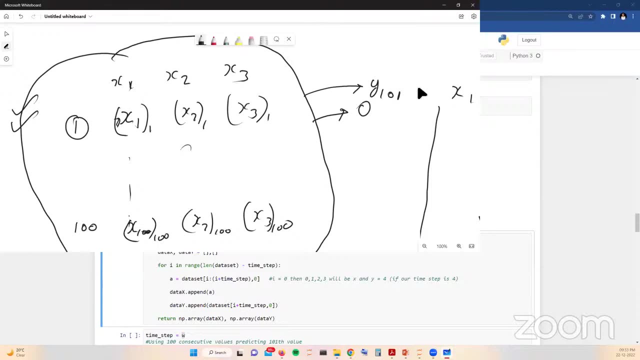 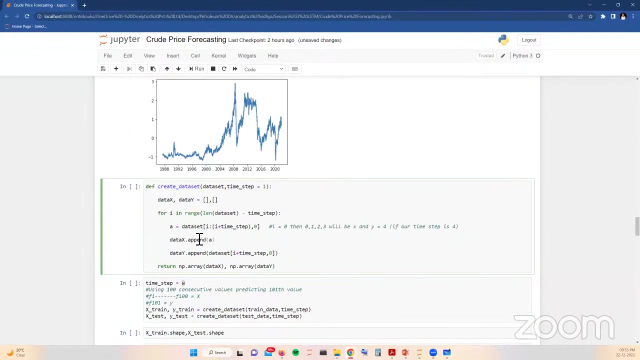 filling the 101th day of data, right? so this particular thing that we saw here- making the batches, this particular thing- first 100 days with 101 day, next 100 days with 100 second days- that particular thing is done here by using just a simple for loop itself and you. 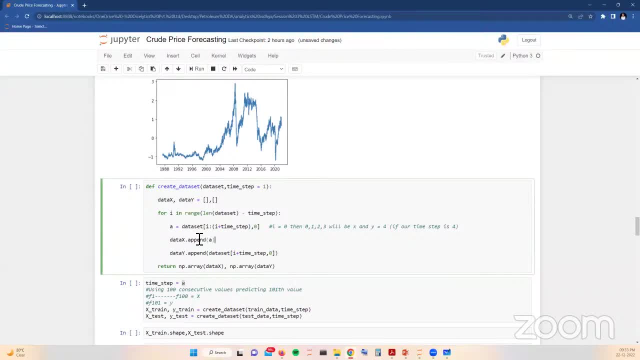 can also do this particular thing by using time series generator that is present inside your tensorflow library itself, but I prefer to do things by my own. that's why I have written this function itself right? so this function will make the 3d data for me for. 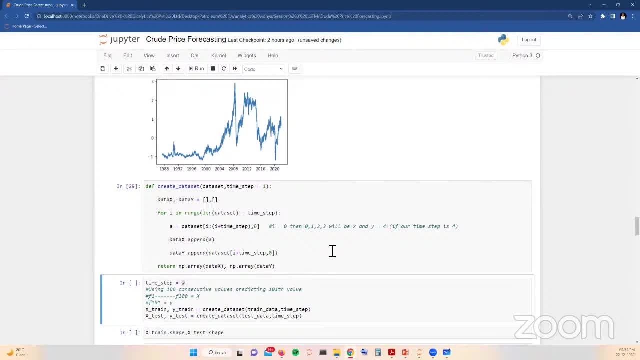 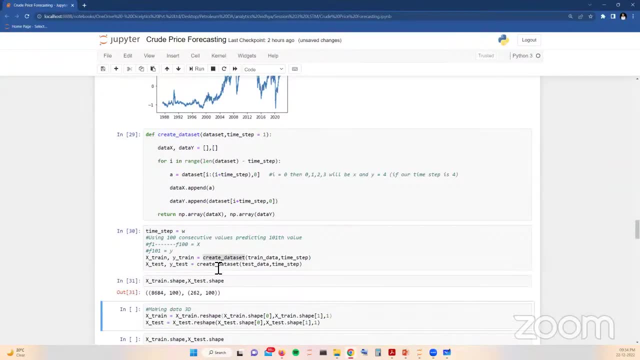 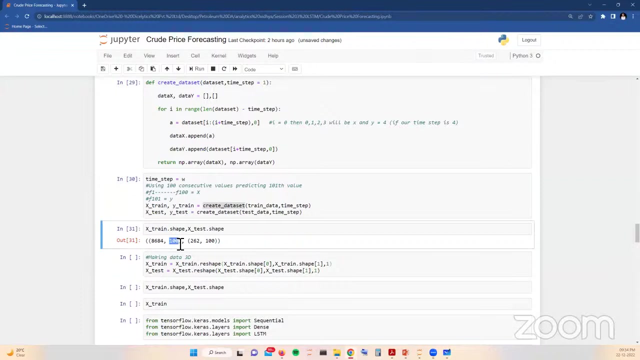 3d batches of data that I need to feed to my LSTM, right? so I am just using this function here making my training set and testing. so now, if you see, shape of my train and test has been changed. now these 100 are there. this why these 100 are there? because I am telling. 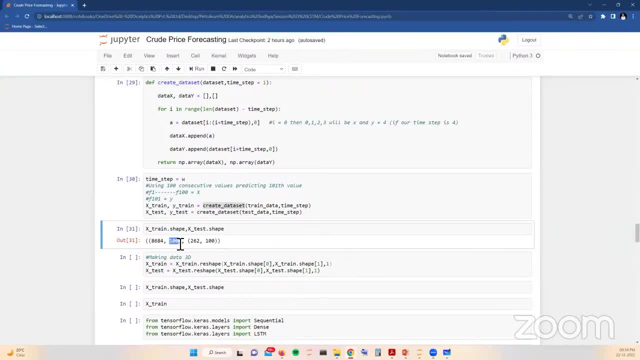 that. further, that first day data is dependent on last 100 days data. so I am just using this function here to make my training set and testing. so now if you see shape of my train and test, that is benefit so kind of in the in the form of様 spot model which I put. 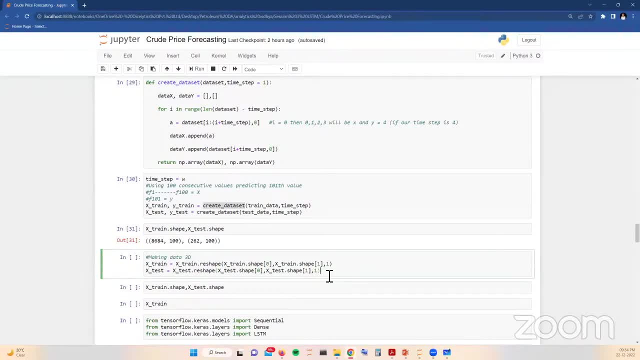 this as before and that changes importantly by 3d, diferen Meeting Rigify. So I am just done that particularly nobody, nothing else, and as in my LSTM 3dhed with requirement 3d, type of structures by just reshaping features waiting. one new dimension here, of one this: 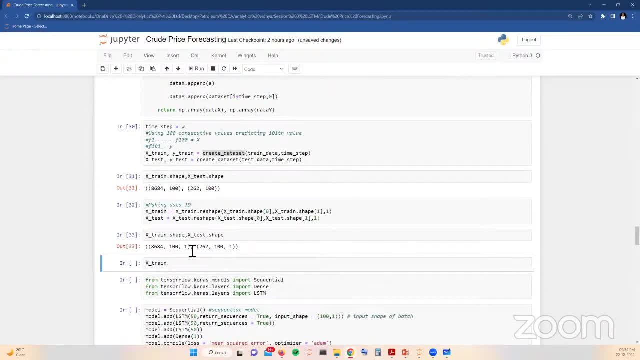 last dimension photo, this last legation. if you see this shape of in this chain, what does this particular shape signifies? So these are the training and definitely training showed that we generally freedom, even though element represent how many total number of features are present in our scenario. as i said, 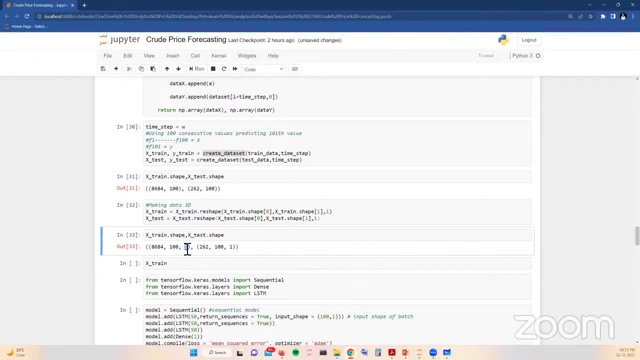 it is a univariate problem. so only one feature is present, that is our growth price itself. but again, if we talk about that machine example, that compressor example, in that particular scenario three features will be there right, this particular thing is representing what window size i am giving. 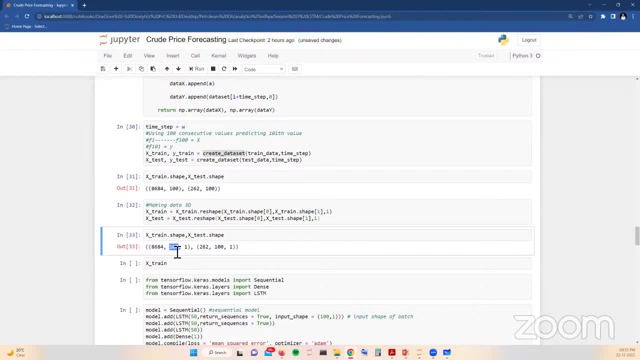 what window i should be. why reshaping is done? the reshaping is basically done because, uh, currently i have only one feature right, but generally lstm expects an input in a 3d structure. so if i have more than one feature, let's say if i have three structures, then i need not to reshape the data. 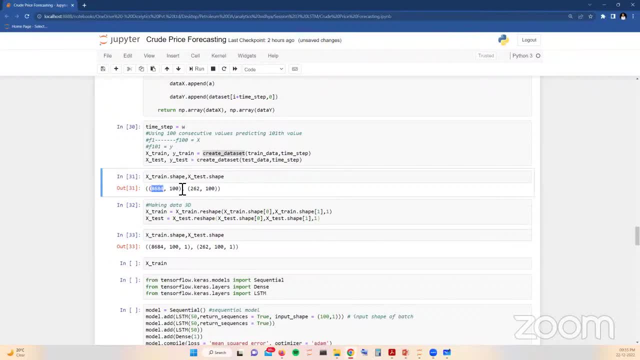 itself. it will automatically, at this time, step itself at this particular time itself, it will automatically. had given me a 3d array here, but as only one uh, i have only one dimension right, one variable. so i need to get uh or i need to shape my array in that particular form itself. 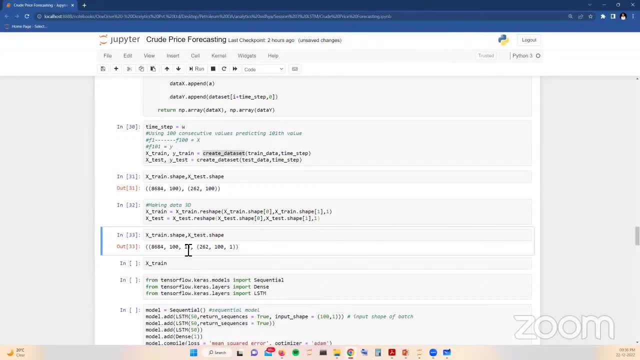 so that lstm understands that. okay, i'm getting a 3d structure, because lstm only takes 3d type of data, 3d arrays only 3d dancers, whatever you, and but when this one will be present here, it will understand that. okay, this is a univariate type of situation. the last dimension kind of tells me. 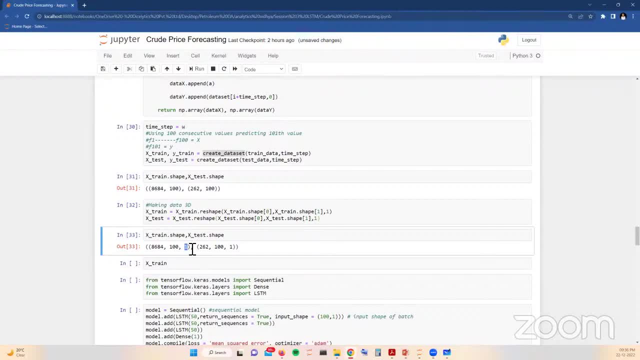 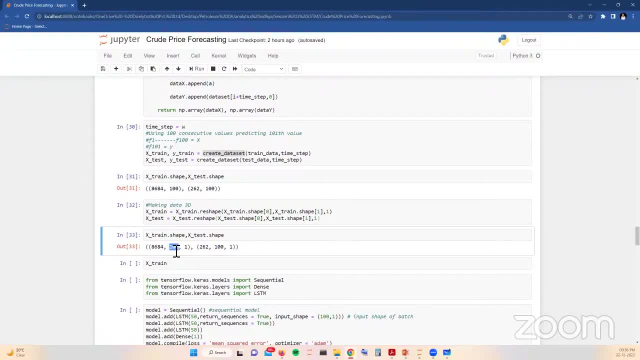 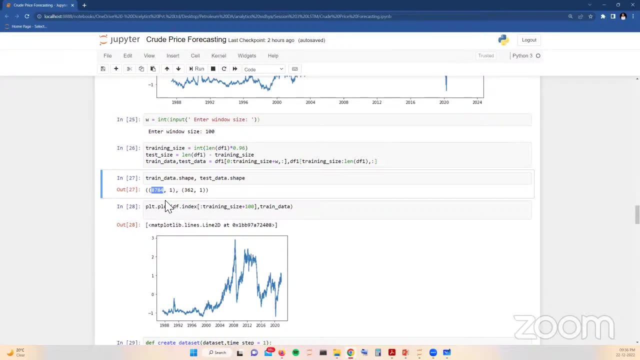 window data. i'm taking 100 days mapping with my 100 right and this particular thing is just calculated by this 100 thing only. for example, if i go above here, you can see my training data. my total training data was 8784 right. 8784 of those were there for my. 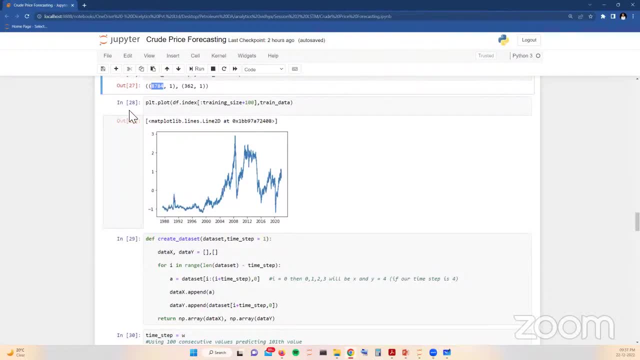 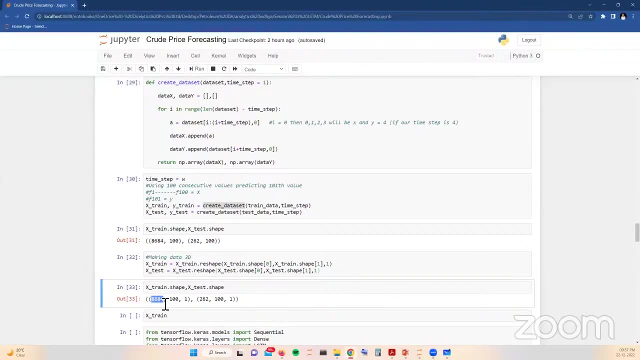 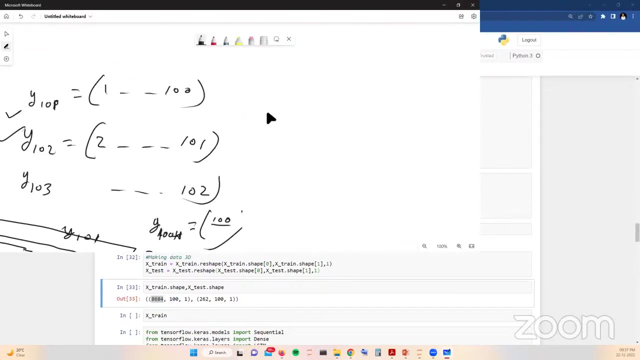 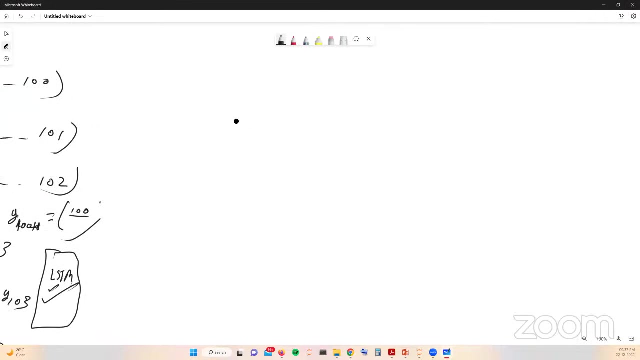 But when I made that particular data in form of this 3D structure, it has been reduced by 100.. Why it has reduced, Let me tell you again. So if you let's take five, let's take five, Let's say: 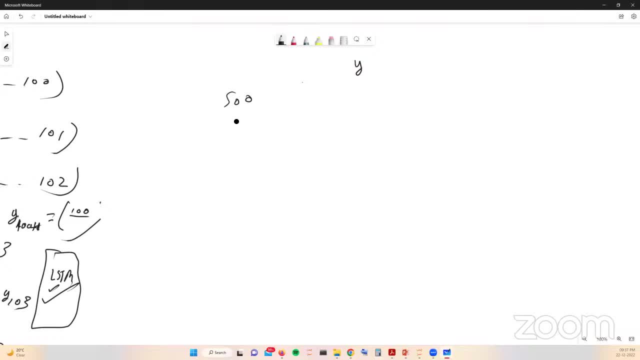 Okay, This is my variable, y or x, whatever. I am having 500 values here, Y 500 starting from my y 1.. And I said I am making 100 days of data, right? So what exactly I am doing? I am taking first 100 values- y 1 till y 100, and I am making 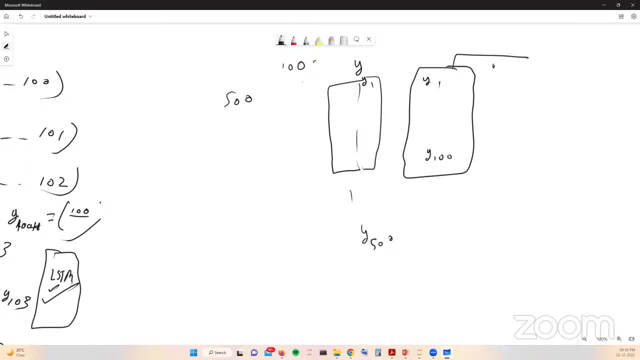 a batch of it Now. my next batch will start from my y 2 till y 100. And this way it will go on. My last batch will end at y 401 and y 512.. Now, if you see, and if you use some of your mathematical logic, how many total number? 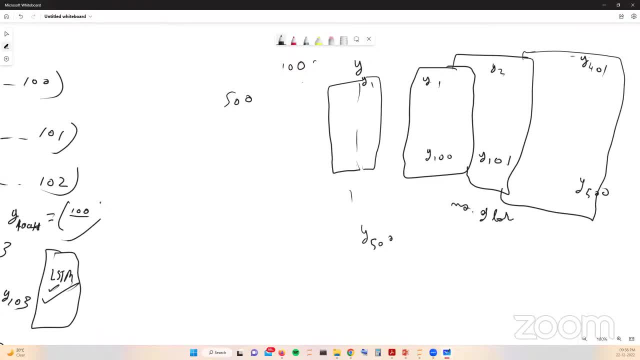 of batches will I have? Number of batches will I have? So I will have total 400 batches, right? If you see it started from y 1 and going till y 400.. So I will have total 400 batches And in a simple way, if you just calculate that initially, I have total 500 lines of data. 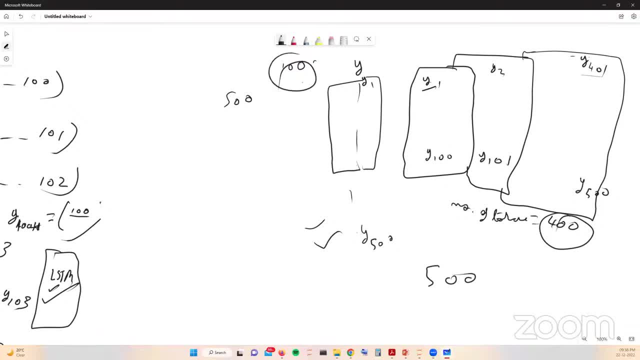 I am making a hundred days of time window. just subtract it, subtract this particular thing, and you will get total number of batches that will be 400.. So this first dimension here is representing your total number of batches. 3D batches that we have. 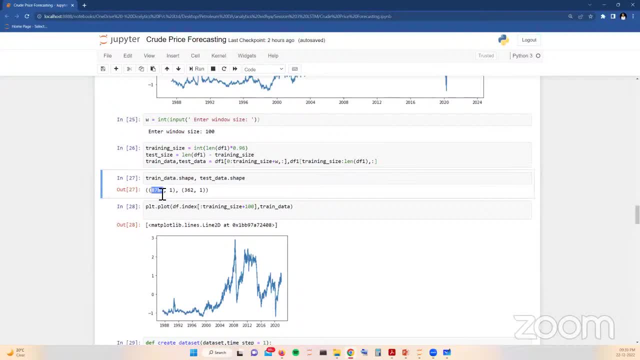 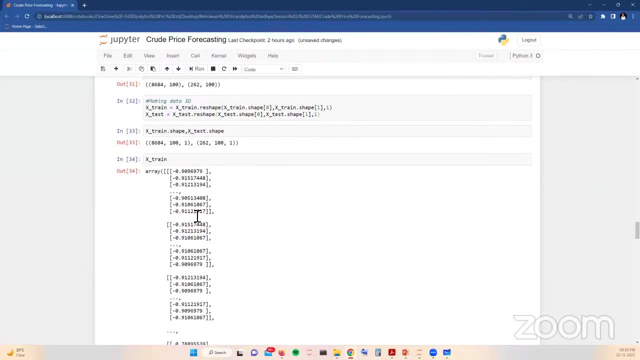 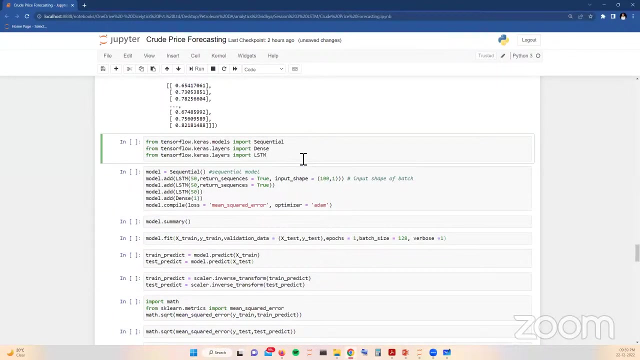 So that will be your 8684.. That is your initial key, That is your initial training data minus 100, right? I hope this is clear to all. So this 3D batches has been generated. now just for let's, just for TensorFlow and from: 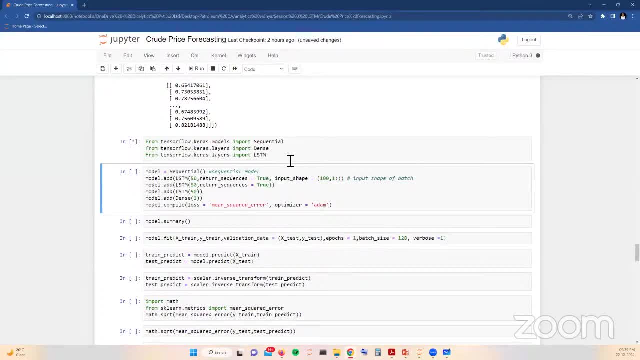 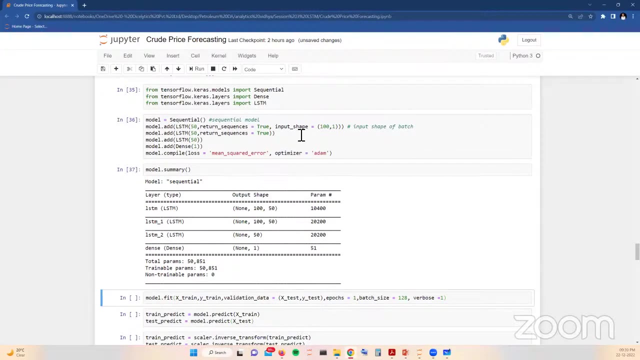 TensorFlow. I'm calling LSTM sense. also, Let's make an architecture of my model neural network model by using these LSTM and Densel. I'm using sequential API of TensorFlow for making the neural network. So it is currently looking like this Input shape: I have mentioned 100 cross 1.. 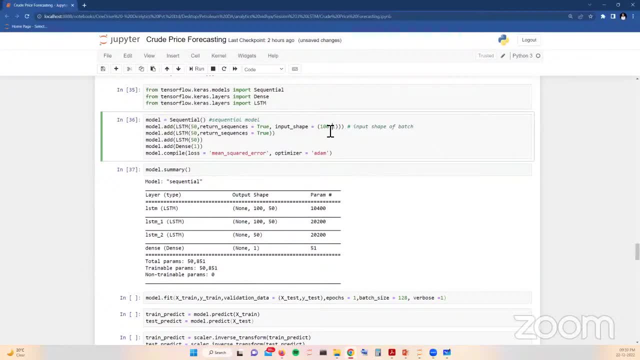 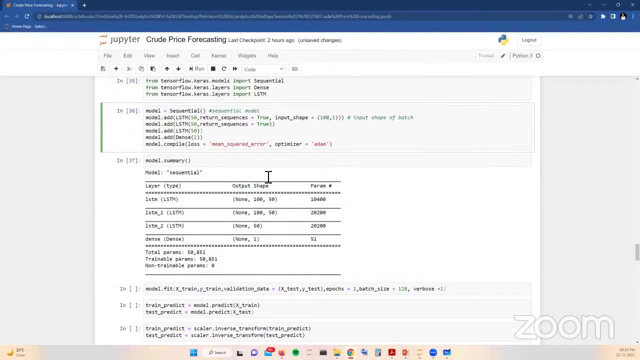 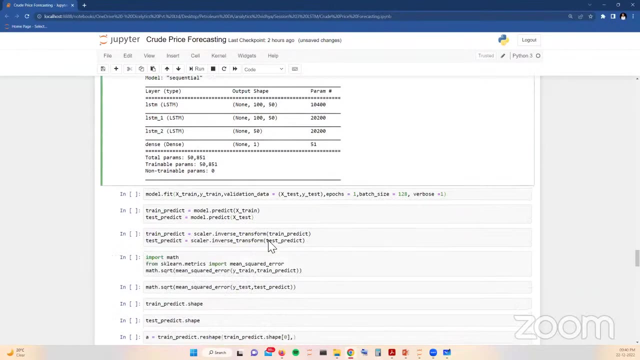 Why 1?? Because I have only one variable price, 100 because my windows was set as at 100.. So 100 cross 1 will be my input shape, Using my loss function as mean. squared error optimizer is Adam, and let's go train our model. 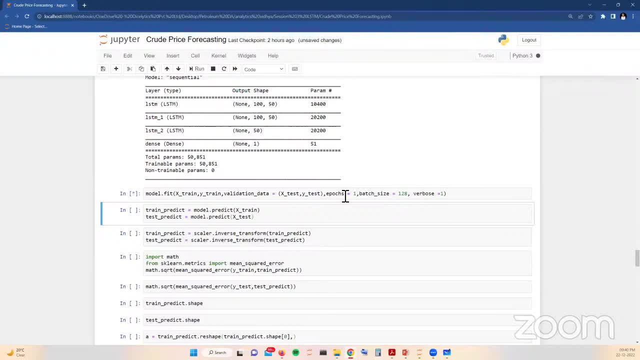 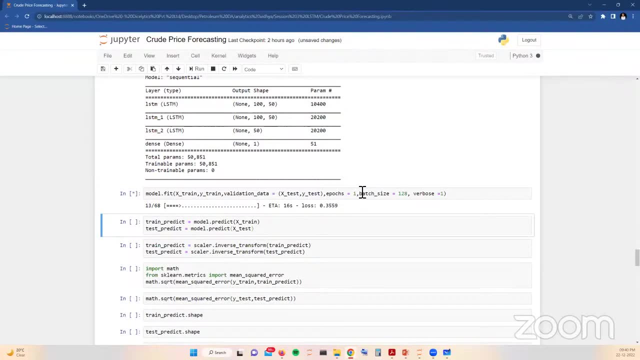 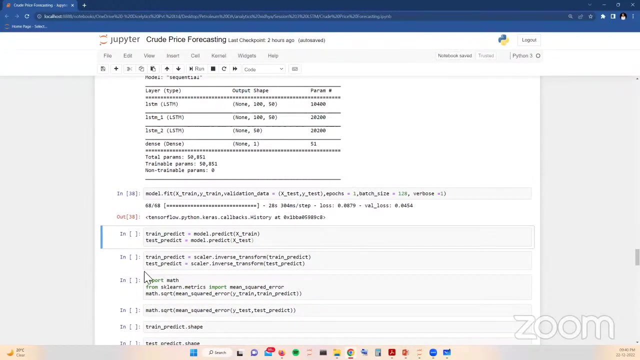 I'm just using one epoch because it will take a lot of time for training. Let's just train it for one epoch here. Ok, Yeah, Model is trained. Now let's predict our next train and next test. Right, let's run the predictions and see how good our model is, straight in when before. 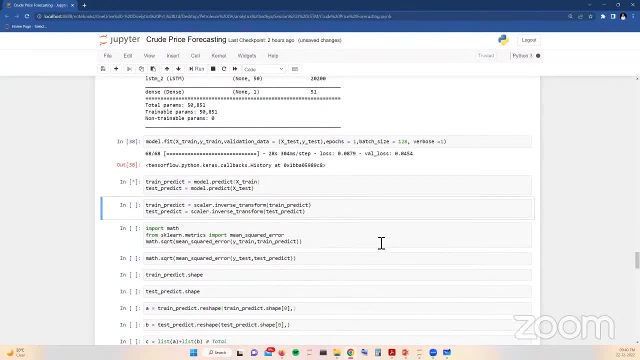 obviously it will give me very bad results, but yeah, let's check it. so i'm using inverse transform because my output from this prediction will come in the scaled version. right, because we have scaled the complete data. so by using inverse transform, let's get back to you, let's get them back to the original shape and let's see what is my mean. 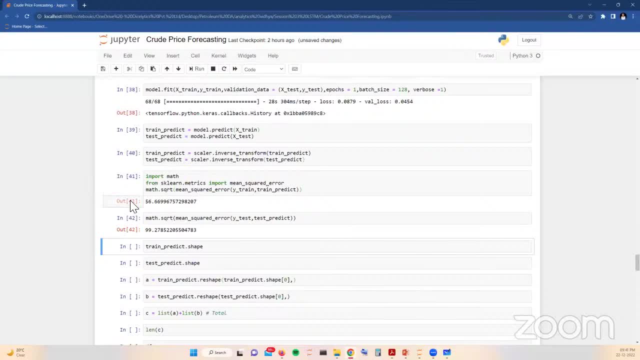 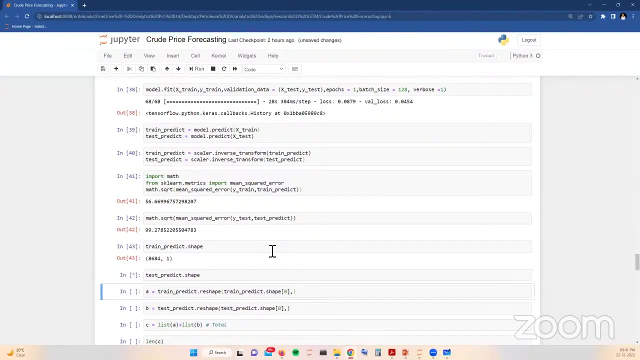 squared error. so my mean squared error for my training part is 56. for testing part is 99. yeah, it is bad, but not that bad compared to my that, compared to the condition that i only trained for one evening, right? so this was my training, said: uh shape, this was my testing. 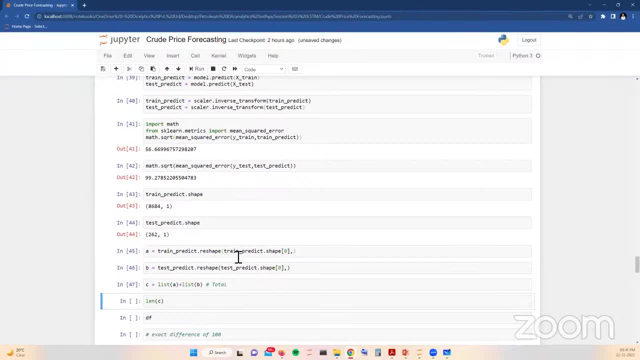 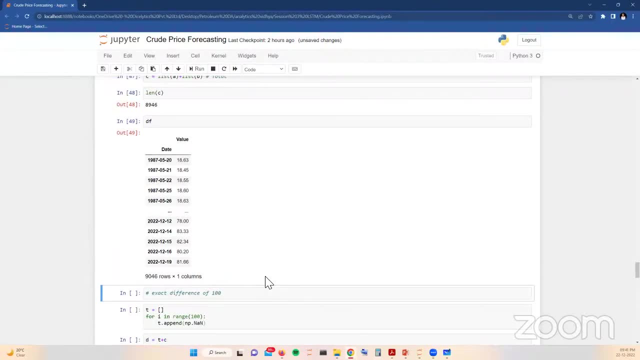 shape. let's make a complete data frame out of it. right, hope my prediction is good. so i'm going to run the predictions and first 100 points will be non-values in this particular data point. you know, because the first 100 points we have taken and then we have predicted. 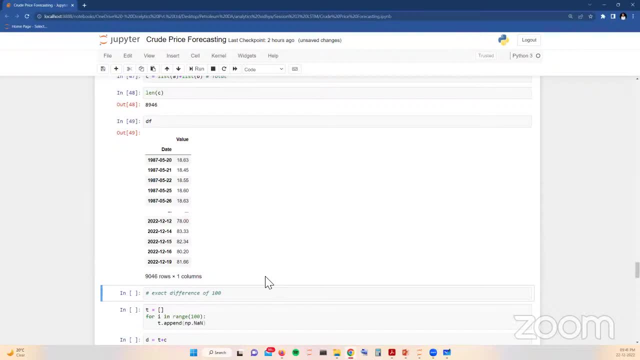 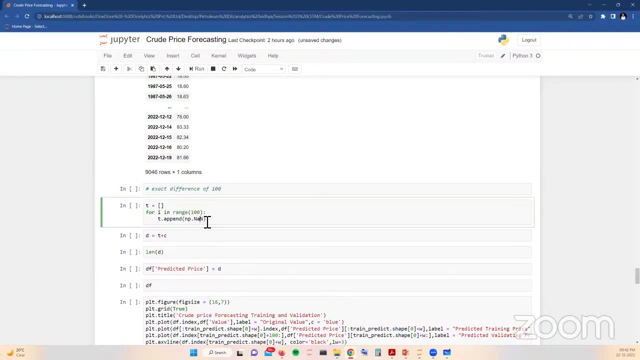 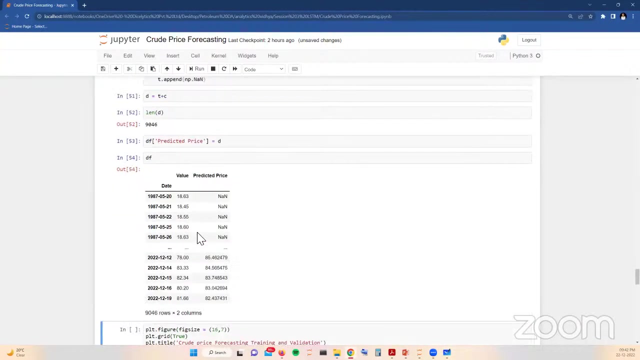 only 101 point, so there is no way of taking, uh getting, the prediction for my first 100 points. that's why there will be non-values and that particular thing- i'm just leaving it here in this one just made by using simple part us logic and python logic. nothing else i have done. 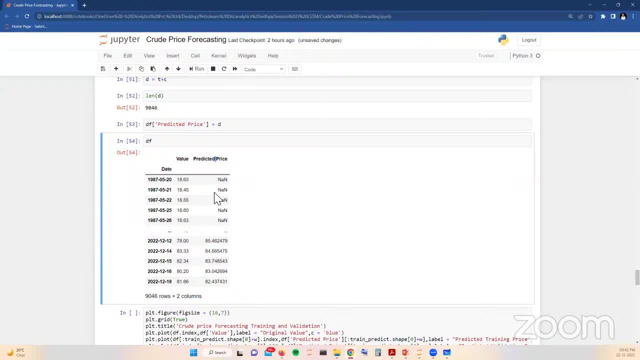 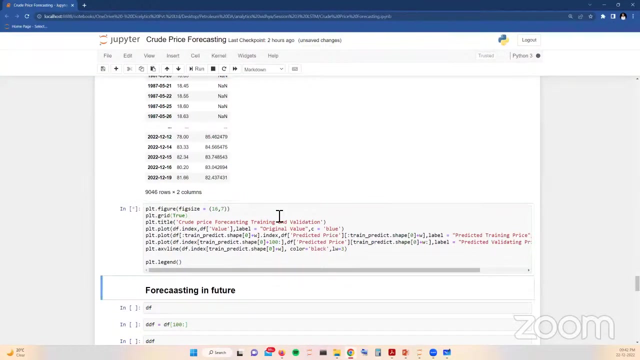 where it will be having the original values and predicted price. and, as i said, first hundred values will be bad because there is no way of getting the predictions for first hundred values right and here just using that plot name for floating purposes, for visualizing, how would my 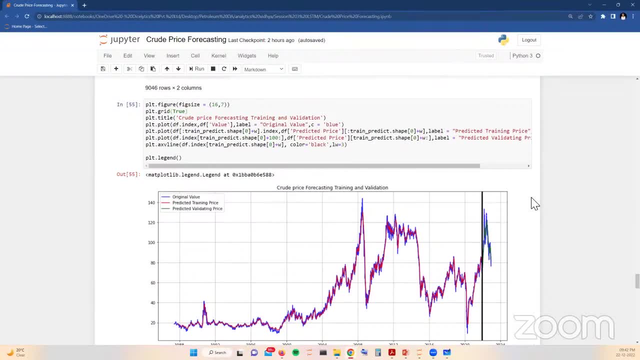 model is straight. so the blue one is my original value, red one is my predicted training price and green one is my predicting validating price or testing price. so till this point, testing we have done. now comes the question: how to forecast in future. that okay, testing i have done. i had the data till 1912, 2022, and i just just have done. 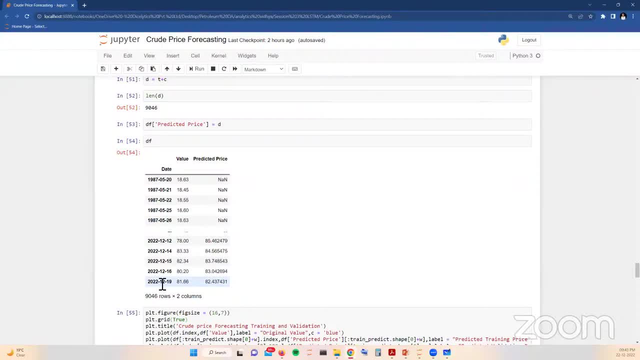 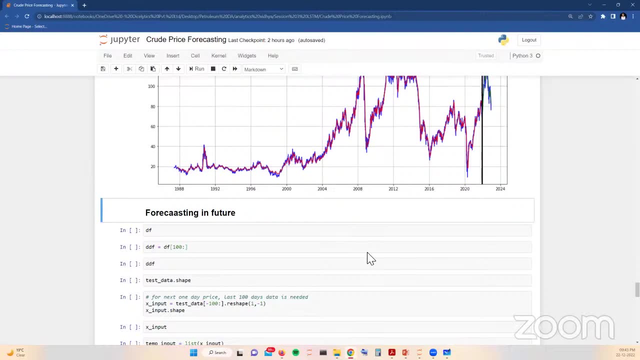 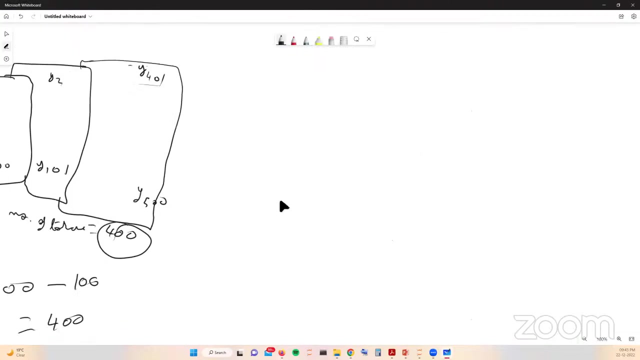 the testing, but how to predict in future, in future, how to predict 20 days in future, 30 days in future, right? so let's see here again, let me open my whiteboard and use the logic, but except there are two ways, right, i'll tell you the way that currently i have used. 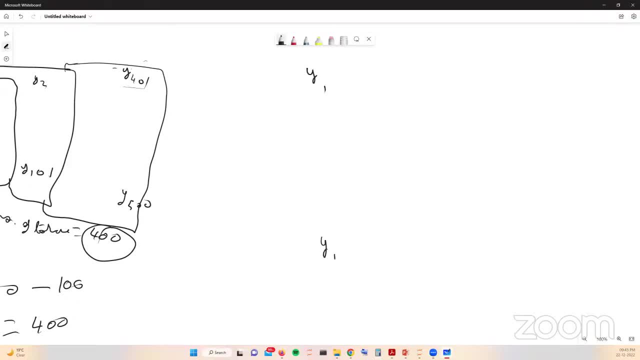 so let's again say i have data from five one, two, five, one hundred right, and i have trained in the such a way that my window size is certain. now this complete data will give me five, one hundred one, five one hundred one. this is my model prediction. so now my first day prediction. i got first day. 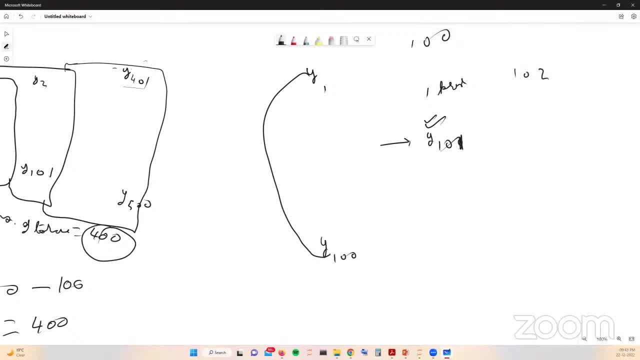 prediction. i got now for predicting for 100 second day. i will take this 100 days, starting from y2, going on to this y100. i will take this 99 days of previous data and i will take the 100 point. this that was predicted by my model itself and i will combine this 100 days data. 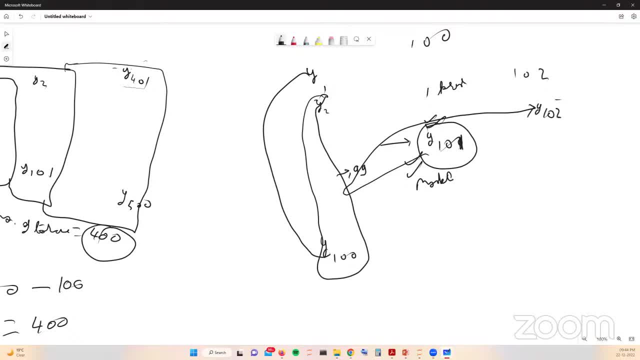 will predict my 500 102. in this way, i will go on predicting my future. but but what is here the things, the thing that come into picture that there obviously there will be some difference between my y actual 101 and my this y predicted 101, and there will be some difference. there will be some error. 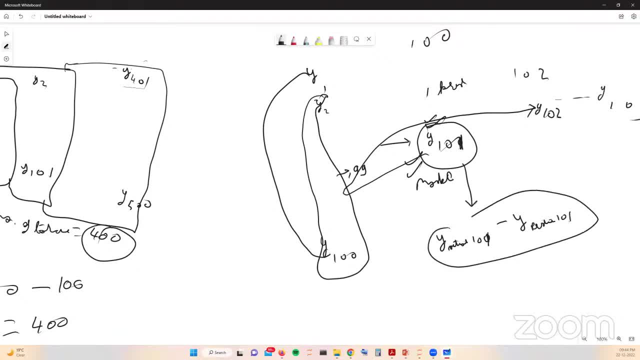 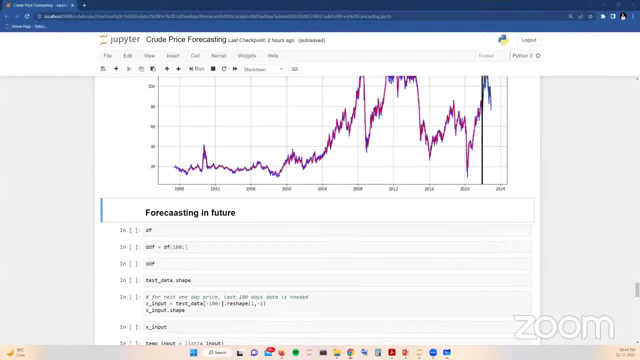 predicted and this error will go on propagation as we go more in future. so this is the program. uh, so sorry for the interruption, but uh, we are running short on time, so i just wanted to remind you that. yeah, just give you two minutes. so now logic is clear, the same logic i've just implemented here. i have taken the last 100 points. 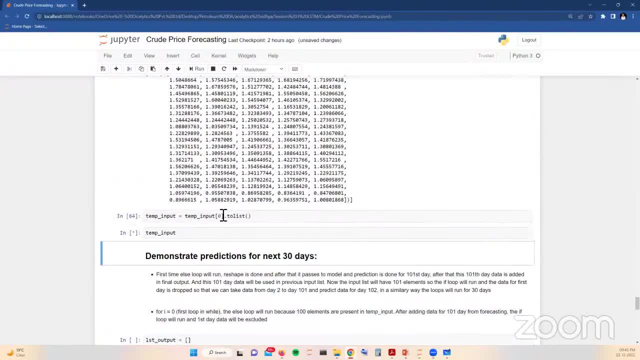 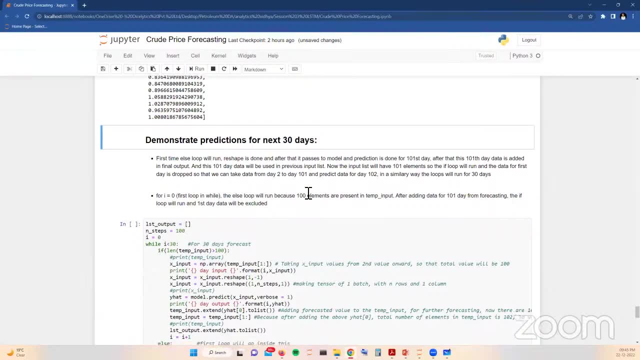 right and from those 100 points taken, these are my last hundred points and from these 100 points the complete, the description i have written here, what i have actually i'm predicting for my next 30 days. so i have just written one if and else loop. 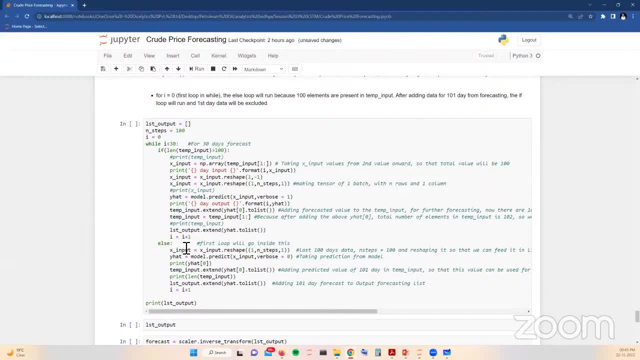 my first look will be this, else no, this cells loop will run and will predict my 100- 130 data and, after getting the 101 day data, that 101 day data and previous 99 days data will be taken inside my if loop and it will predict for my 102 days in this way. so, talking about different, 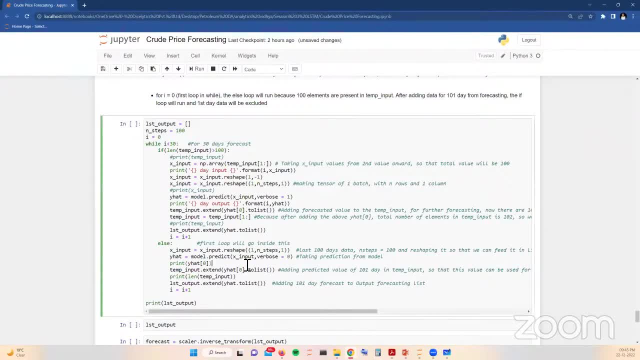 types or from the details of the last hundred points. i am predicting the present one and an if and the next two rents, dono, the wind data and the data was predicted. i practice the next 30 days days. in this way, i will be able to predict for my 30 days. let's run this cell, get the output. 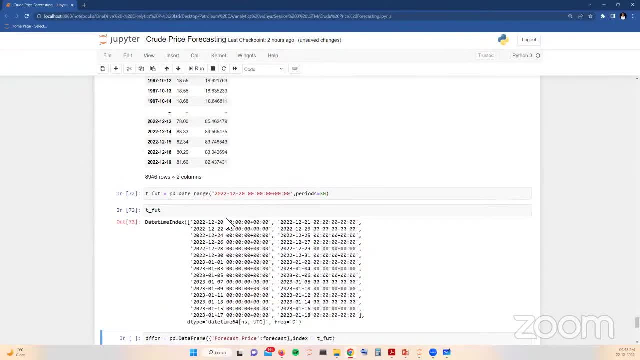 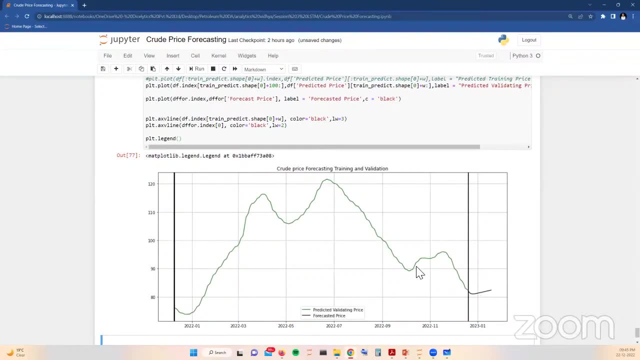 so this is my output here. now again, i'm just using simple part tasks and here, if i show you my prediction for the future, this is my forecasting value. this, this is my, this is my testing value. you can see here that it is kind of getting some of 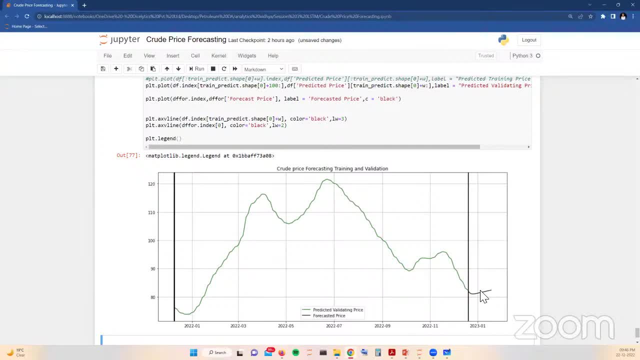 the trend that, okay, your oil price will increase in future. right, so this was the implementation and, sorry guys, we had some of the time constraint. that's why i was not able to give you complete code walkthrough. but, yeah, let me share the github link with you guys. 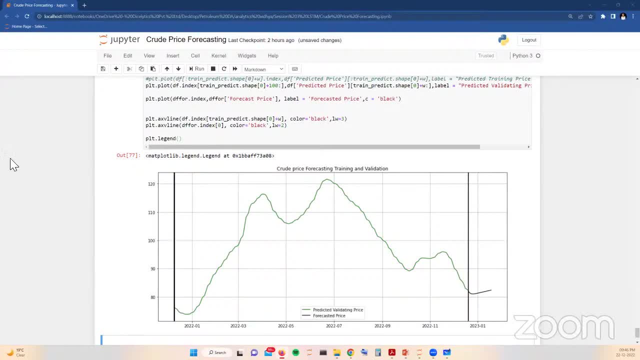 so this: this is my github repository. here you can find different, different projects and let me share the repository. this is my github profile where you can find different different project and let me share the repository where i'm going to update this particular project itself. so i'm just sending this guys. so, uh, this one, this particular one, is where you will get this.